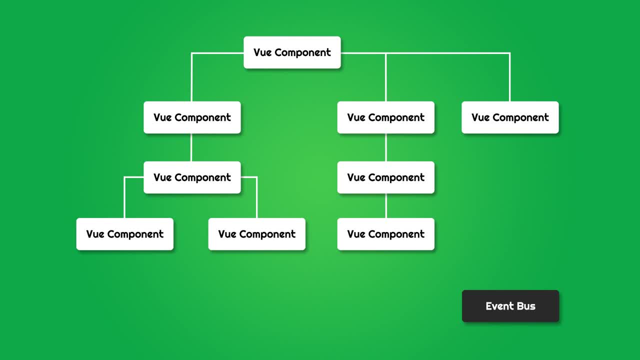 So, yeah, it's better and it's all you need for mid-sized applications. There's nothing wrong, it's a nice valid tool. 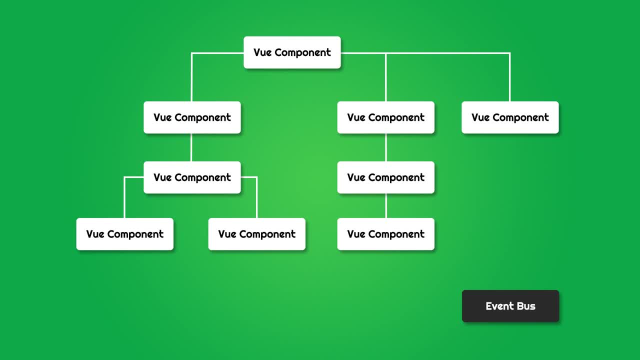 But for large applications with many different component layers, it might not be the best tool. You need for this case a different setup. 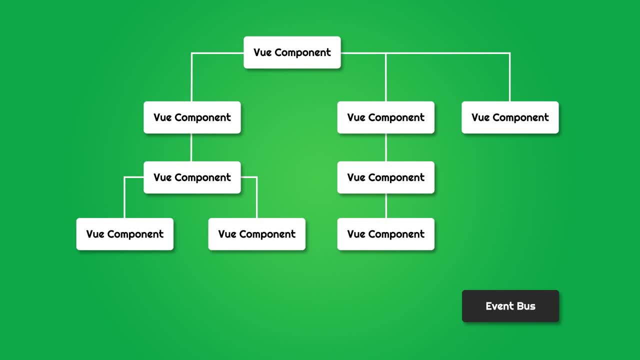 Where you have a unique or a central place, you can store everything and a place you can define your way to change data and to get the data. 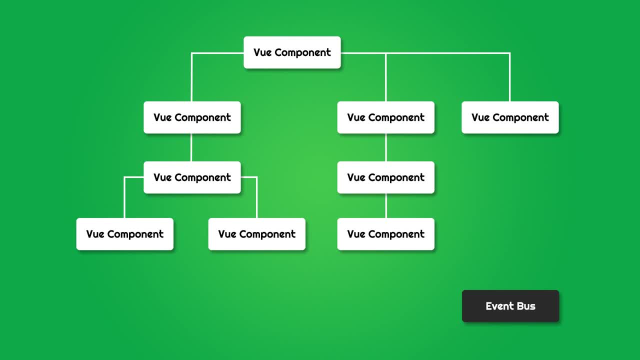 So, you have a really clear separation of concerns and you can easily track the changes on your data and so on. 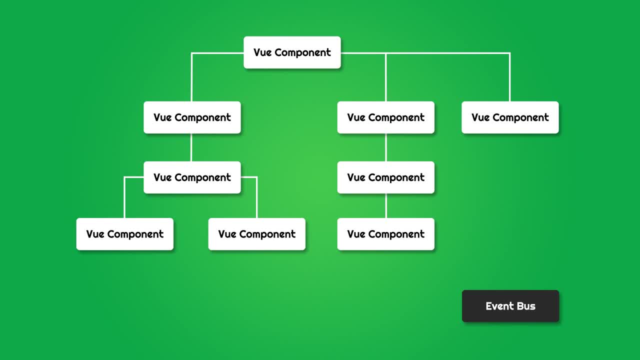 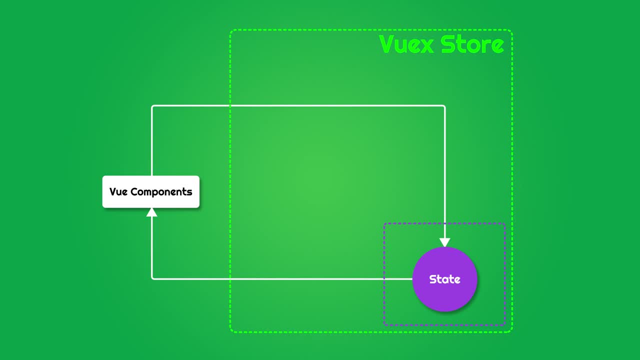 UX will offer you a pattern for this, so let's take a look. The UX pattern or library has the idea of using a central store, where your state is stored. And that is the key. You have one file in the end, where you store the application state. And that does not mean that your components cannot have their own state. When you have data or properties in a component, which is only used in this component and only changed in it, there is no need to put this data in the UX store. 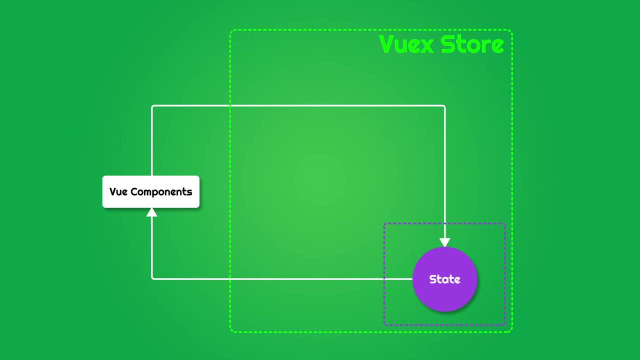 But everything which you use in different components or places should go in there. With such a central store, you could access it from every component and change it, and then on another component, you can simply access it to get the data. 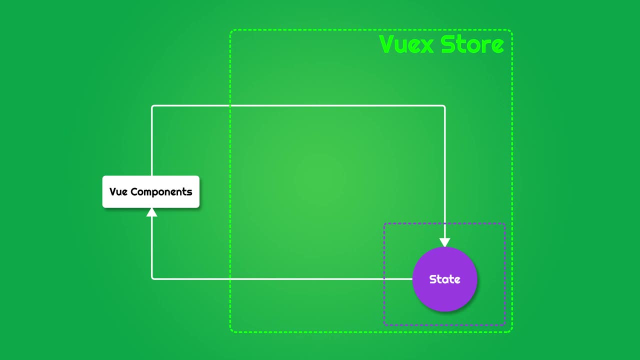 Ok, now, how you can use the UX store. Now, you will see this here in action. 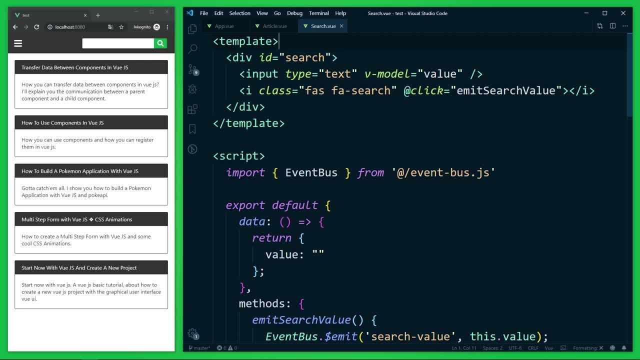 Ok, I have opened up the project from the last tutorial with the event bus, and I would like to rebuild this project and add the data. So, let's create the UX store as a central state. 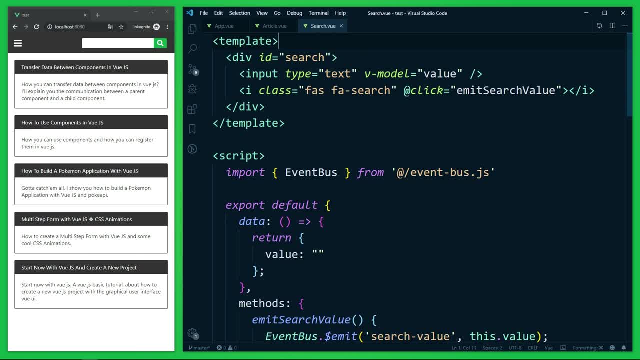 If you have not seen the last tutorial, I link it in the info card. 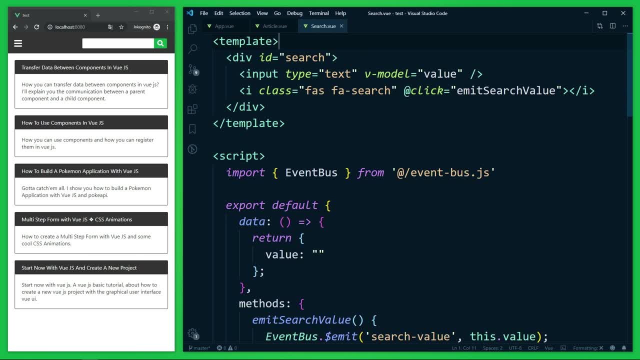 First, you need some helpers from the Vuex package. 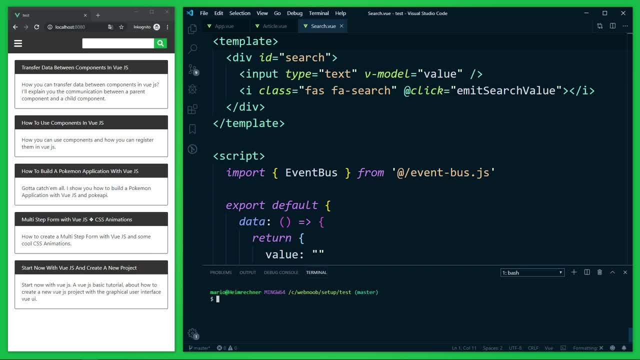 So, let's install it with npm install –save and then Vuex. This will download Vuex. 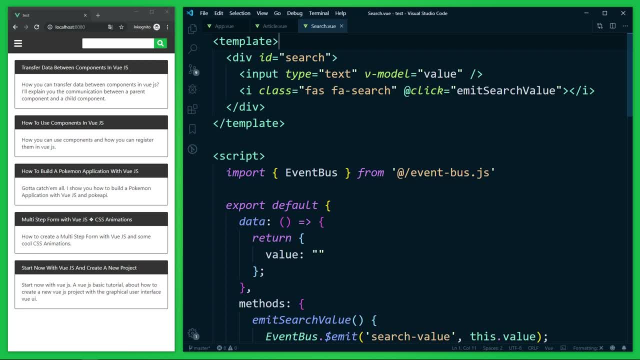 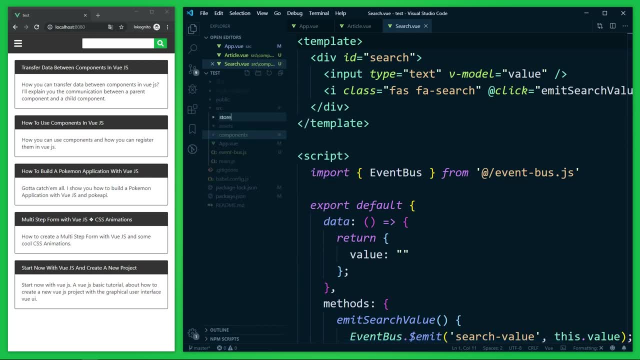 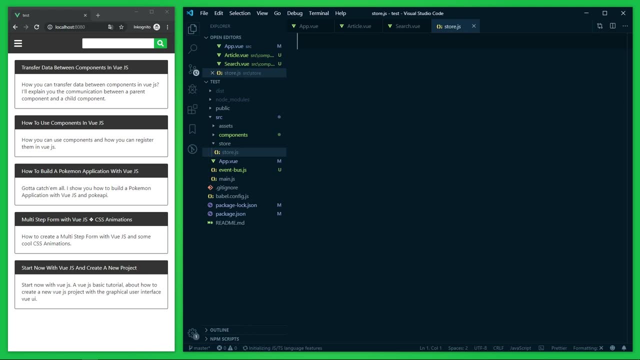 If it's finished, you can use the Vuex library. So, let's create it. I will create a new folder, store, and I will create a new file, the store.js file. Yes, it's a simple javascript file. And here, what you need to do is first, import Vue from the Vue package, and second, import Vuex from the Vuex package. So, these are the tools you will need here. 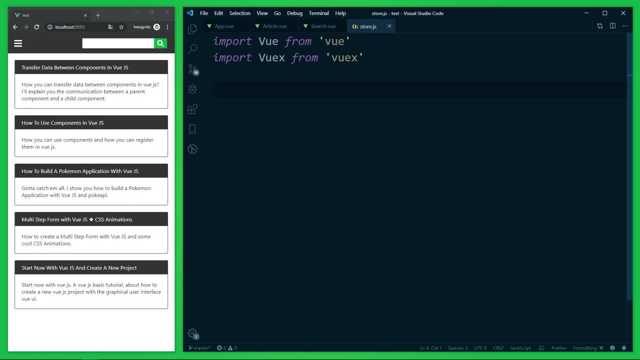 And now, you can simply tell Vue to use Vuex, to register this plugin, basically, right? With this, you enable the Vuex functionality in your application, and here, you can create now your central state and manage them in this file. Let's do this by typing new Vuex store, like this. And store is a method. Where you can pass an object with the configuration for that store. Now, for holding a centralized state, Vuex provides a property for this, named simply state. 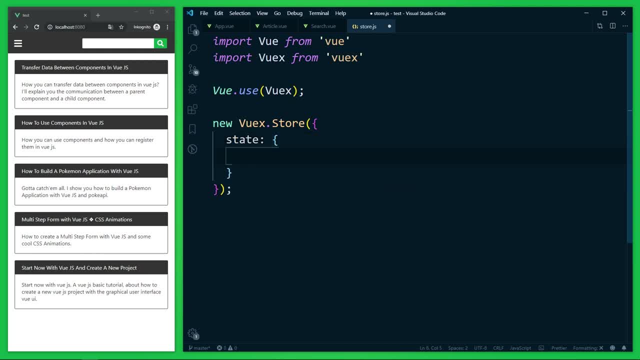 And this is an object where you can define all your properties, like the local data attribute in components. 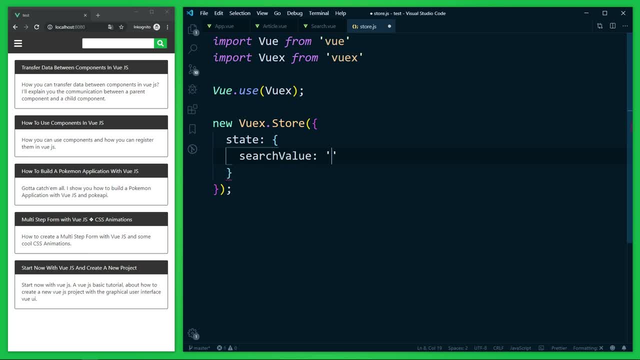 So, let's do this with search value, with an empty string as default value. 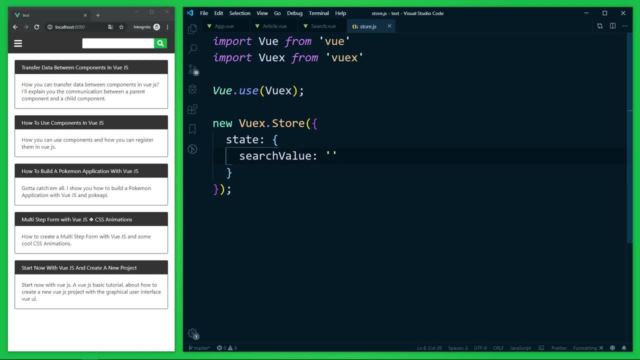 And now, how you can use this state. Before you can use the store, you have to export it first, right here. With export, a constant named store, in which now, the store is saved. Ok, let's stick to the main.js file and import the new Vuex store, with import, store, from the store.js file. In our store folder. 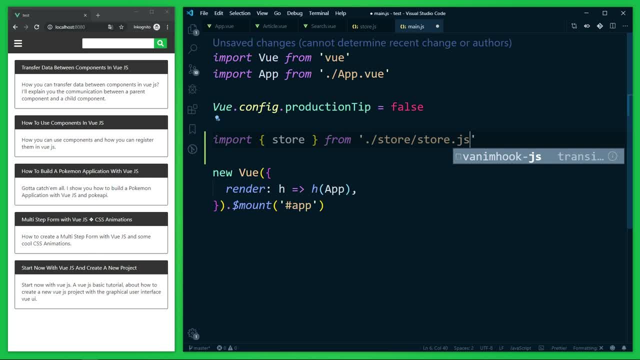 Now, with this, the new store is imported. And all you have to do is register it here as a property on your Vue instance, with simply the store property and as a value, the imported constant, which holds the Vuex store. 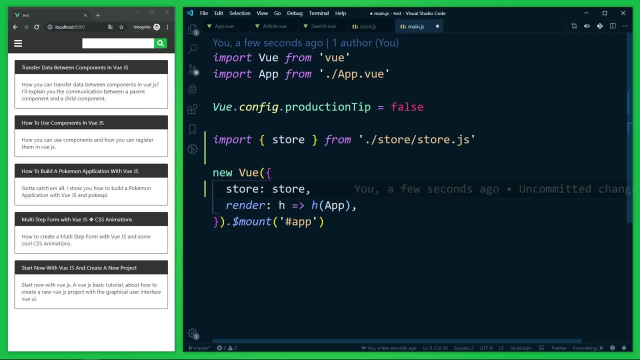 And if you use the same name, you can use the E6 shortcut, which sets automatically the right key-value pairs in this case. 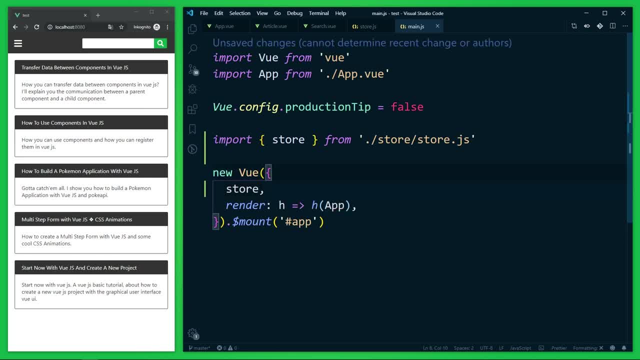 So, with that, the store is now added to your root Vue instance. And you have access to it in all components. 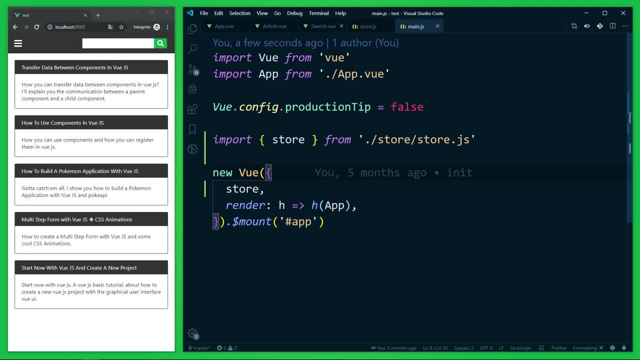 Let's stick to the first component, the search component. And here, we don't need the event bus anymore. 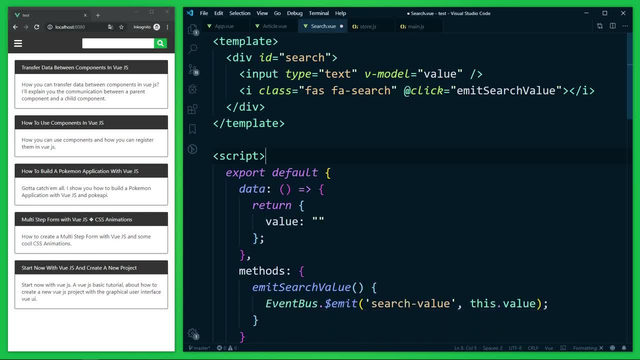 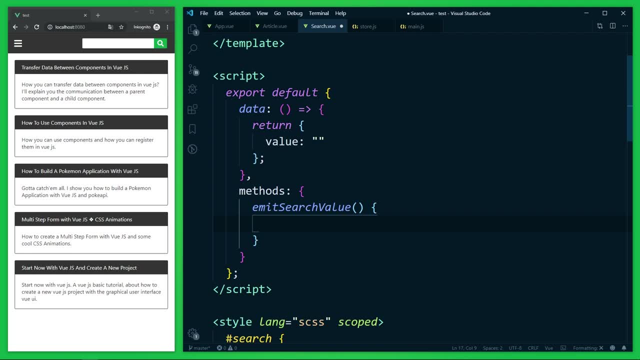 So, let's delete this line of code. And in the emit function, you can also delete this line here. With this, you can now directly access the state in the Vuex store, with this, dollar store, state. 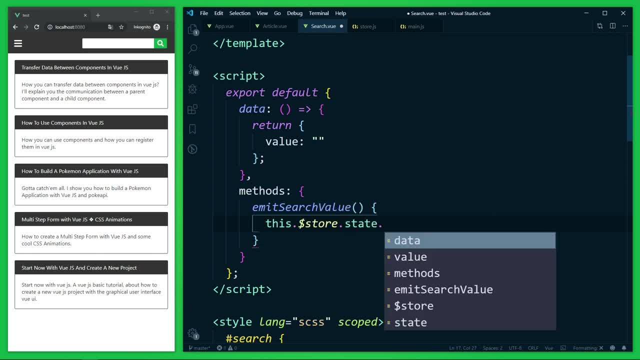 And here, the property you want to access, in this case, search, value. And this property gets the value from the local state in this component. Ok, let's check the article component. Here, you can also delete this. 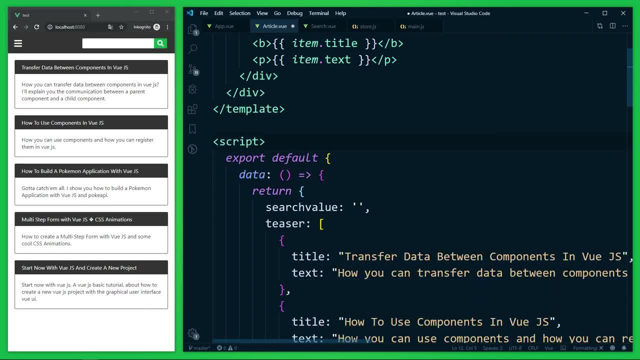 The import, and you don't need the created function anymore. 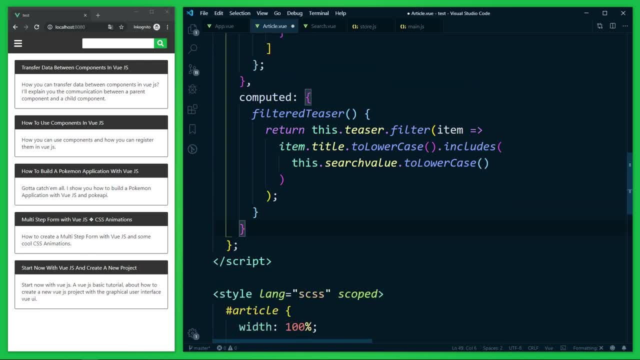 So, I delete this quickly. For your state, can you use a computed property, so let's create one. I call it search value. And here, you can access it as before, with this, dollar store, state, and search value. 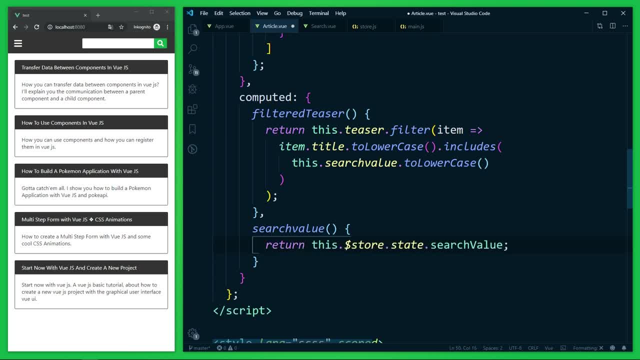 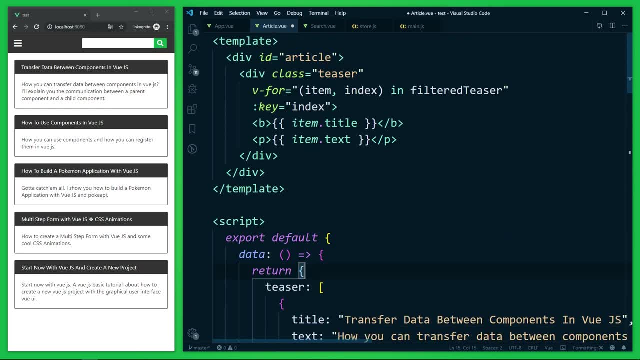 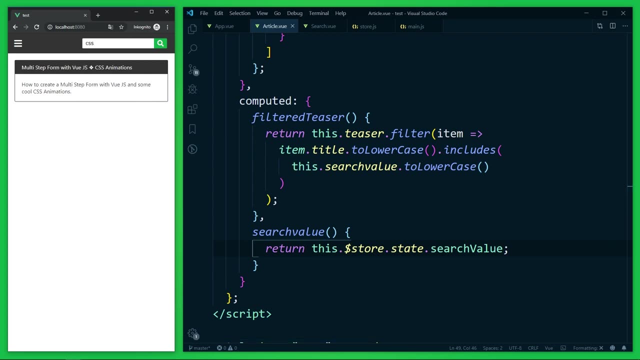 Last but not least, you can now delete the local attribute here. Ok, I save now. And let's check if everything works as before. Yes, it works. That's fine and improved a little bit. 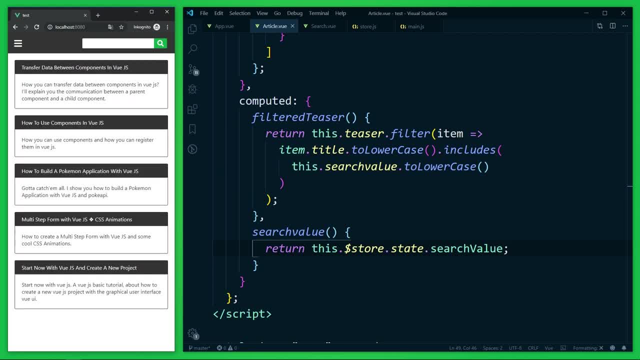 But you don't really have many benefits here, right? Hmm. 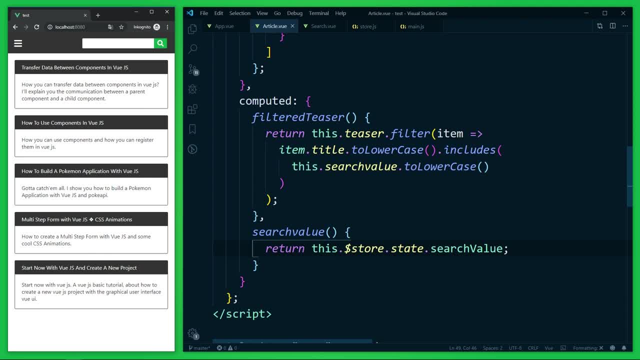 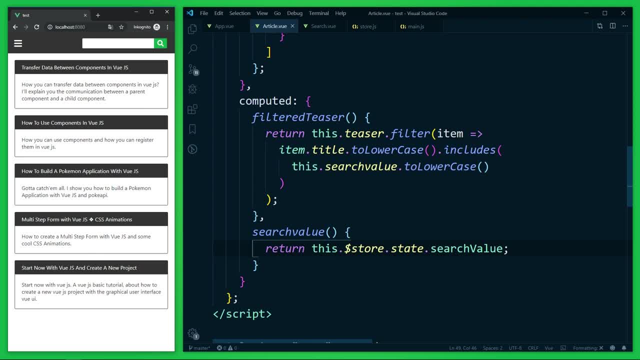 Already is a lot better, but still has some issues. 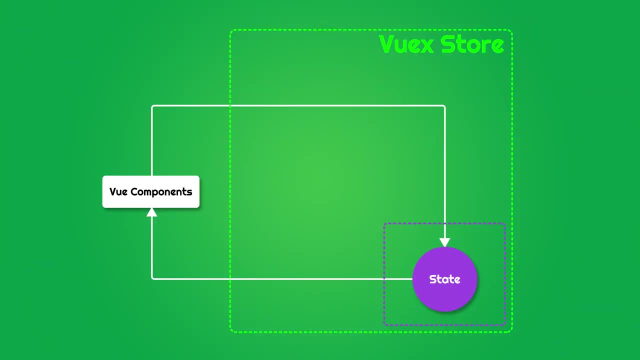 But you can still improve this. Imagine you have more components like the article component, where you want to filter 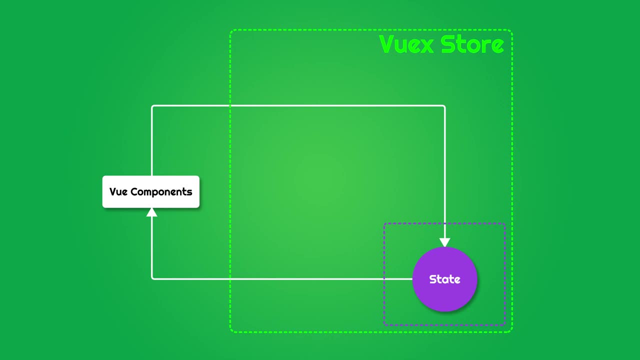 the teaser based on the search value. For example, the issue is that you would quickly face the problem that you have duplicate code all over the place, and that is never a good sign. It does reach its limits in larger applications, where you do more with the state. 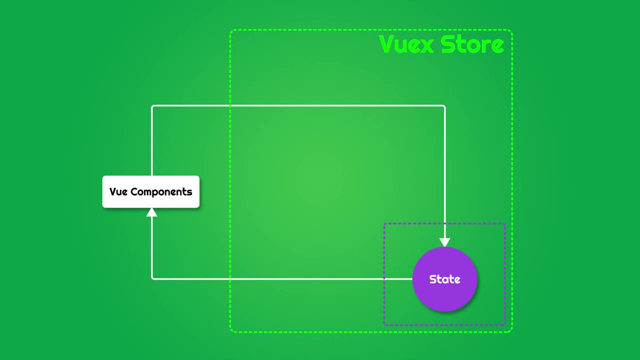 There is a solution to this problem. Instead of directly accessing the central state in the component, where you want to 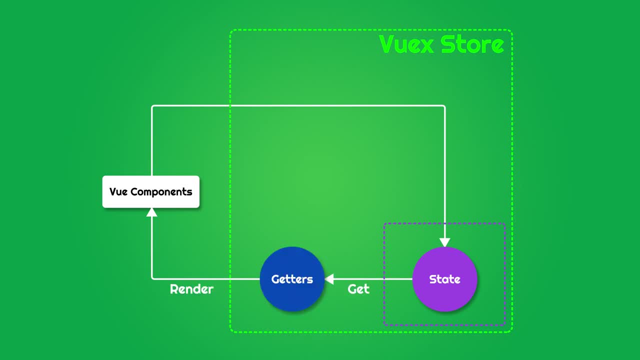 access it, you can create a getter method in your Vuex store, where you can filter or do other calculations. 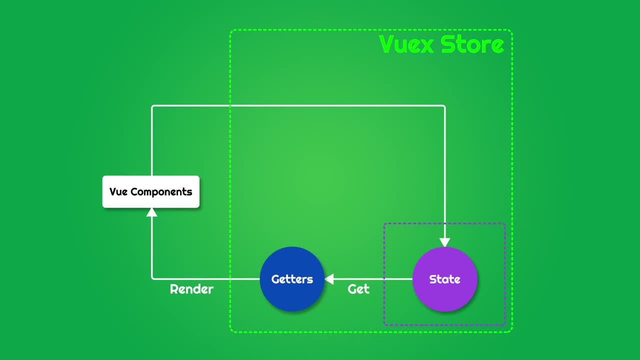 These getter methods are also centralized in your Vuex store. 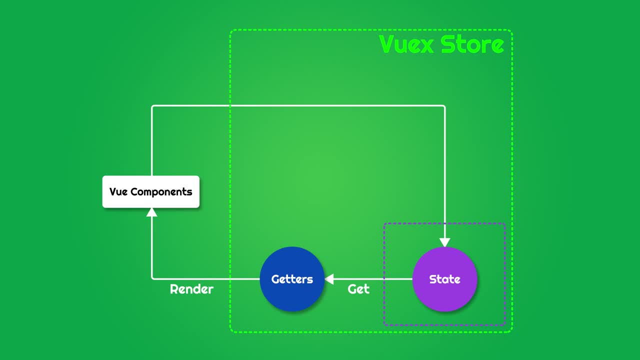 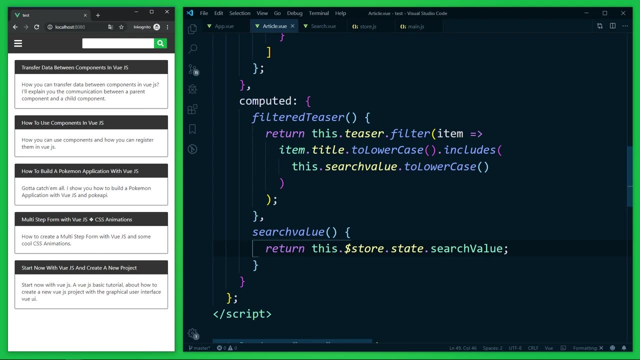 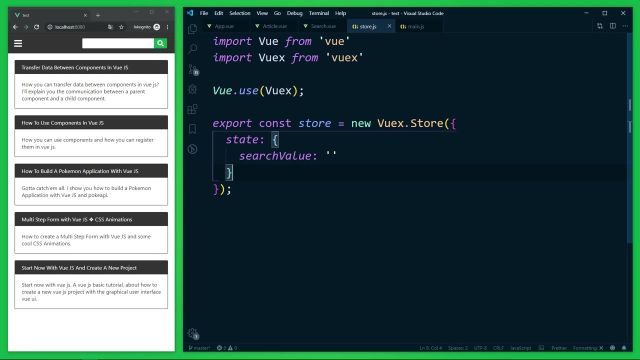 Let's take a look at how you could implement this. Ok, we want to outsource this computed property here with the filter into a getter method. Let's go back to the stored.js file. And here you can now add a new property. Vuex provides a property for this. Called getters. And this is also an object which holds your getter methods. And here you can choose any name you want. 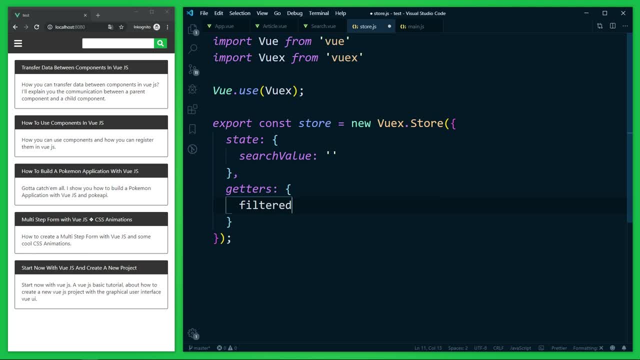 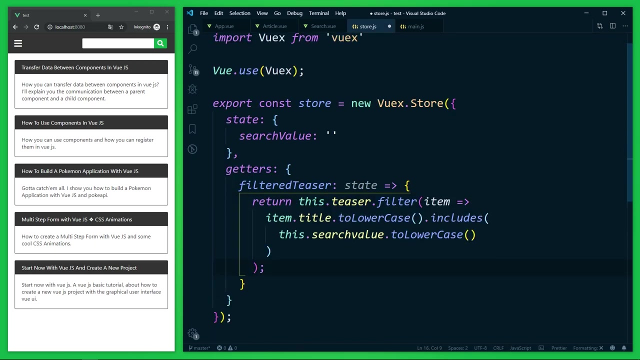 I write filter with teaser. This function gets the state as an argument. This is passed by Vuex automatically when this function is executed. And here between the curly braces you can do with the state whatever you want. In this case is the goal to filter the teaser based on the search value. So let's copy quickly these few lines here. And here you should change this to state. But there is a problem. You don't have the teaser in the Vuex store. So let's put them also in this state here. 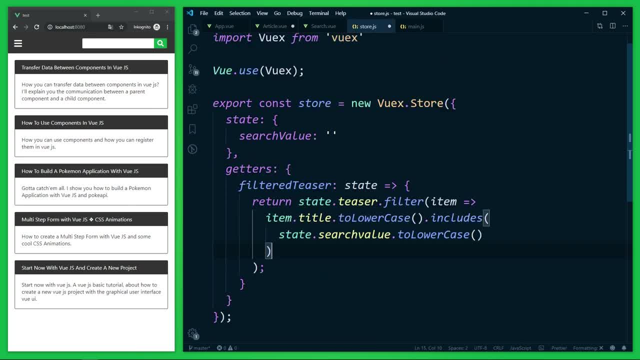 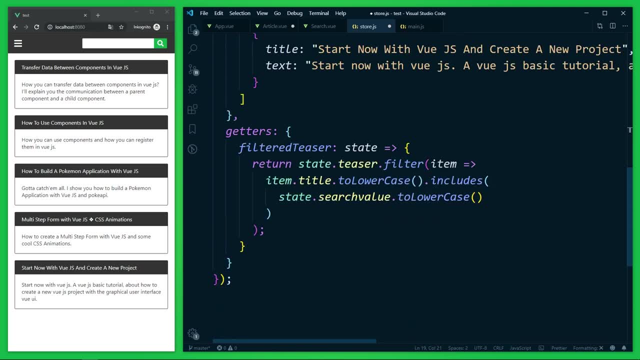 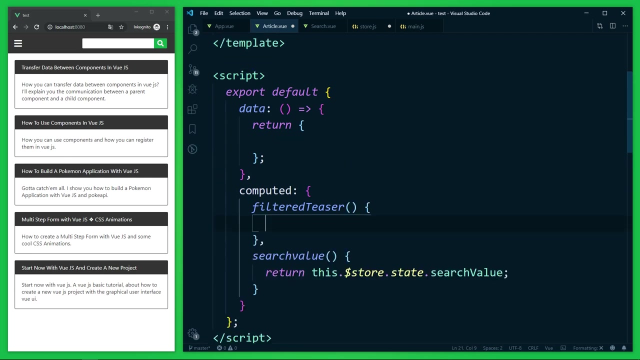 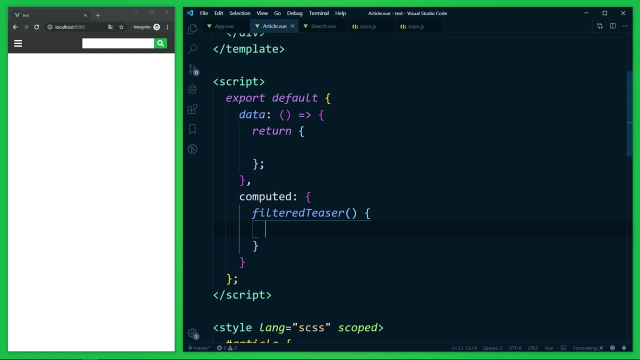 Now with this getter in place, you need to access it in your components, right? So let's stick to the article component again and clean it up a little bit. Things you don't need anymore. And here I reused this computed property. And used the new getter method. With this, dollar store, and getters, and the name of the function you want to execute. Filter it, teaser, but without the parentheses. You don't execute it though, Vuex does it for us automatically. 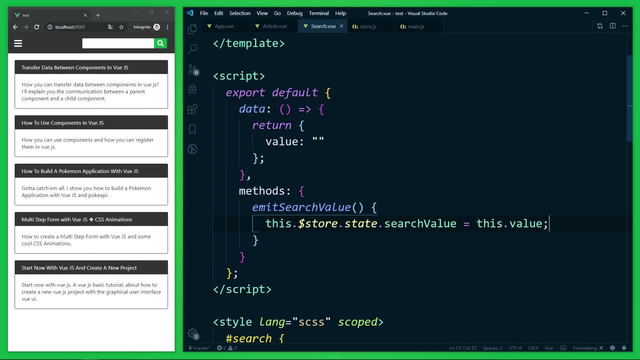 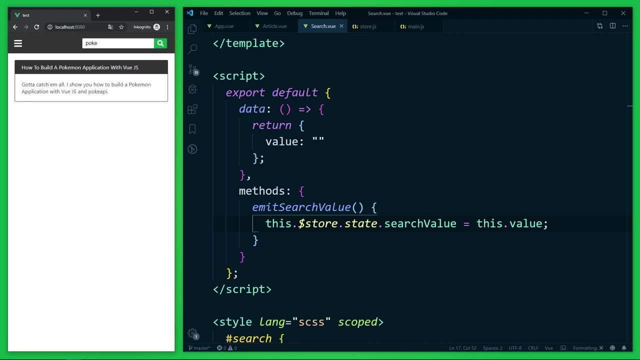 Ok, time to save, and you see, it still works as before. But now you have this logic here decoupled with the getter method, which you can reuse it in all your components. 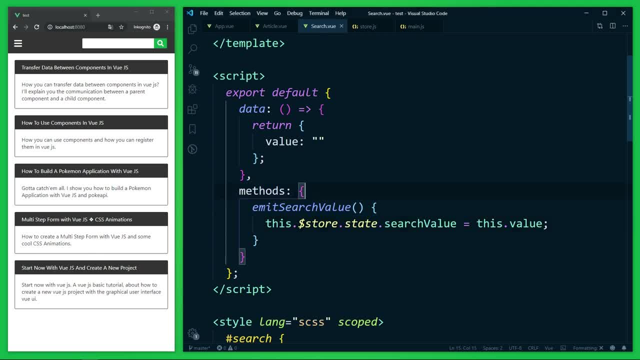 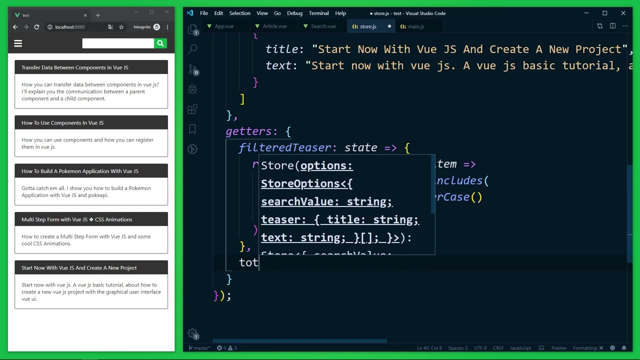 And this is the first awesome benefit you get. You can use this pattern here to outsource your business logic related to your state. But there is a little issue you may have if you create more and more getters. Now, let's say you have another getter, for example. A getter method that returns the total count of all teasers. So, I create this method quickly. 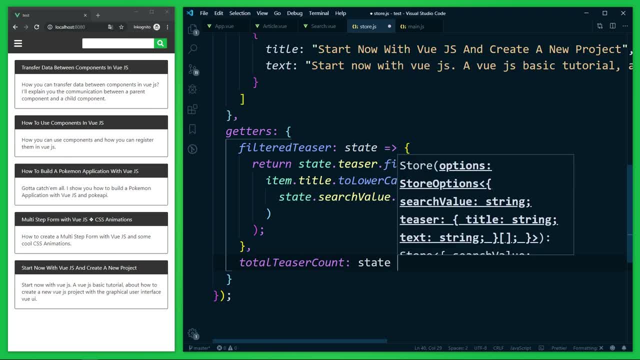 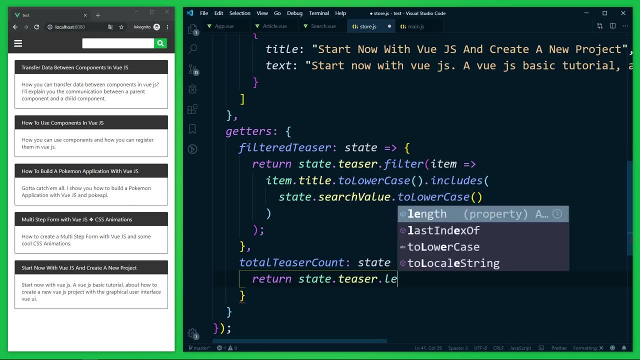 TotalTeaserCount. With the state as an argument, and here I return the length from the teaser array. 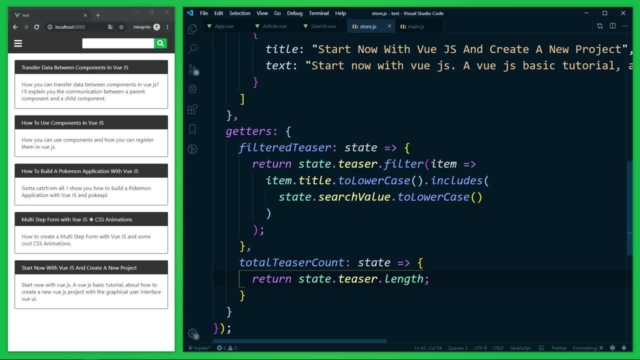 I want to use this getter in the article component. So, let's stick to it. 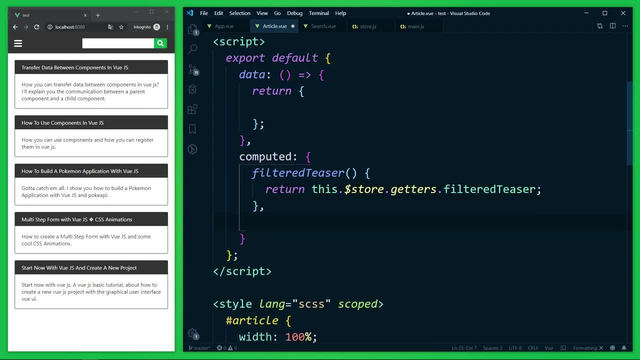 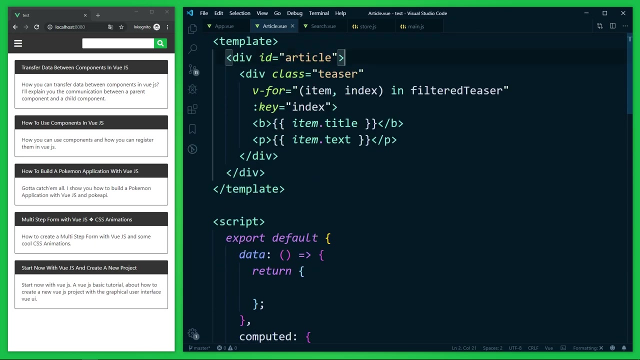 And here I define a new computed property to get the value. I named it also TotalTeaserCount. And here I fetch the value and copy this line here quickly and change the method to TotalTeaserCount. And here in the template section, I want to output this number. So, I create a new div element with a class SearchResults. 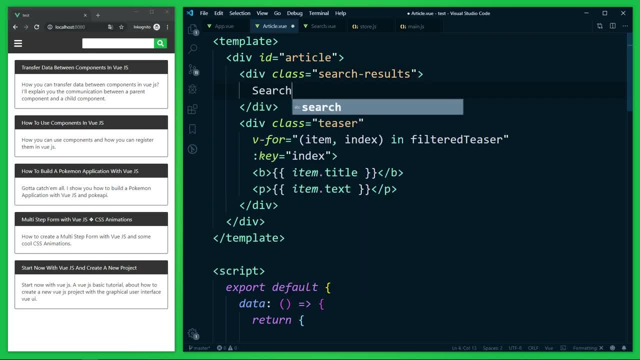 In there, I want to output some text. SearchResults, for example. 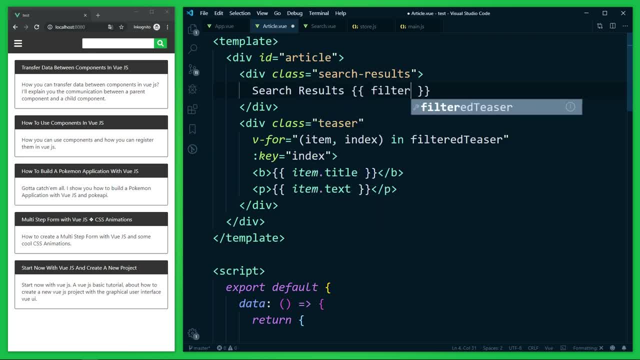 And now the length from the filtered teaser. And here our total teaser count. 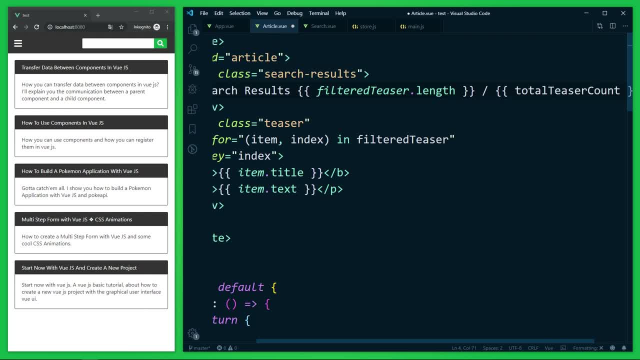 Let's quickly give the new CSS class some style. Just for the look and feel. 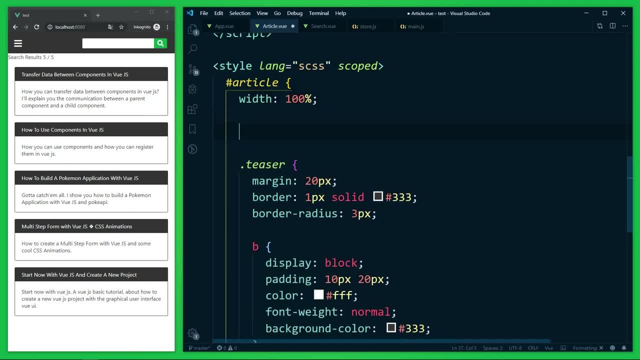 Let's say 20 pixels to the top, the right side, zero to the bottom, and also 20 to the left side. 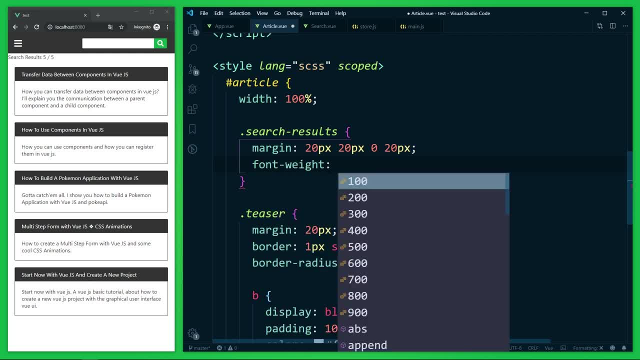 And let's show the font on board. Time to save, and let's see if it works. Yeah, it looks good. 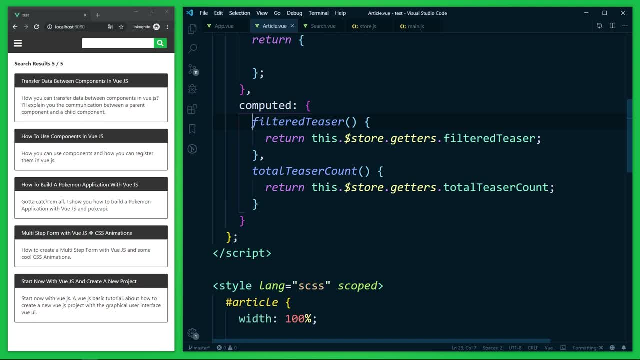 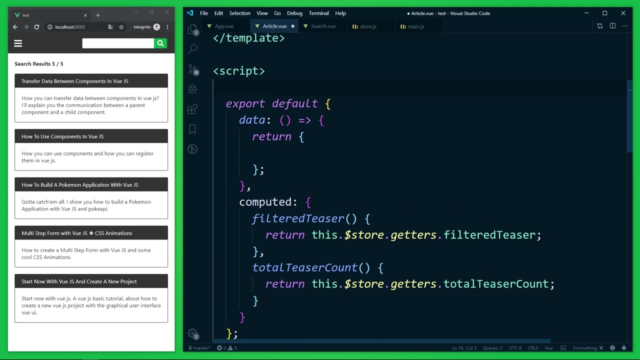 The problem is that you have now two computed properties. her to fetch your getters. And if you add more and more getters, you have to repeat that for every getter. That is possible, but it would be better if Vuex would do that automatically and give us access to all the getters without having to set up a computed property for each getter. Well, turns out Vuex has a helper for that you can use. It has a method which will create all the computed properties you need. And if you want to use this helper method, you should import it. 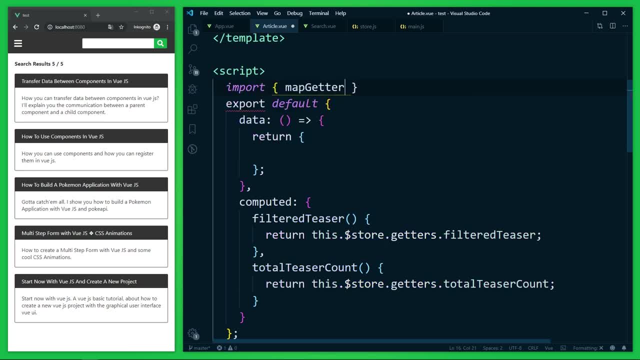 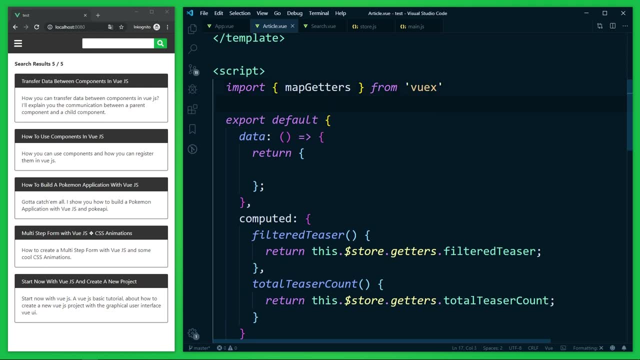 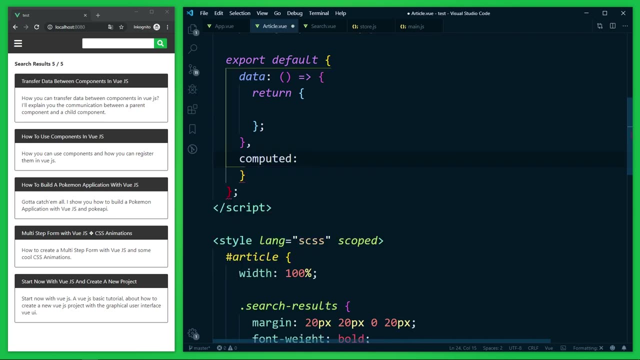 And the helper is called mapGetters from Vuex. And now you can delete this computed properties here and set the mapGetters function as a value. And this takes an array as an argument or an object if you want to map the getters to different names. I use the array syntax and here you can simply specify as strings all the getters you want to use in this component. So for example, if you want both getters, we have right now the filteredTeaser and the totalTeaserCount. That is a much better way to save a lot of code and if gives you an easy way to access your getters. 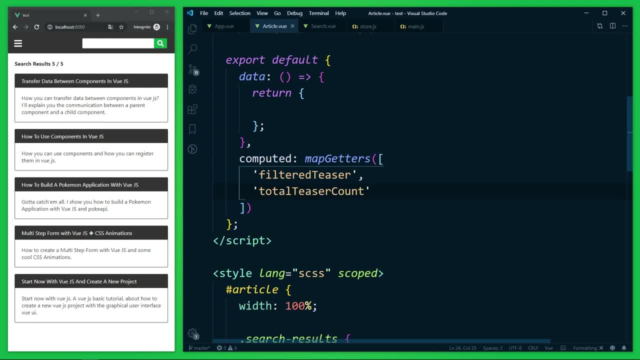 But it has a big issue. Do you see it? 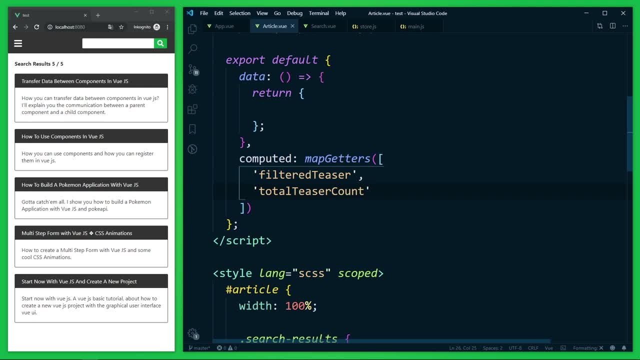 You can't create additional computed properties for something totally unrelated to your central state, right? 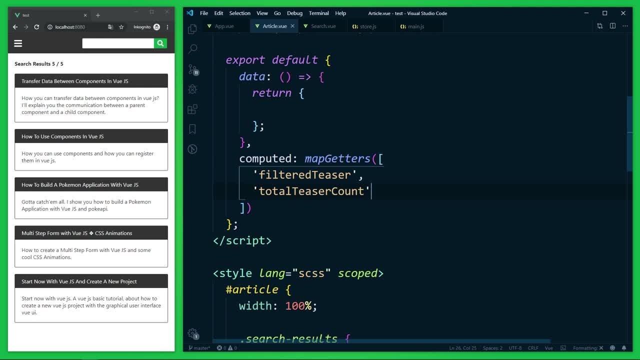 And this is not really optimal. MapGetters here is the whole value of this computed attribute. 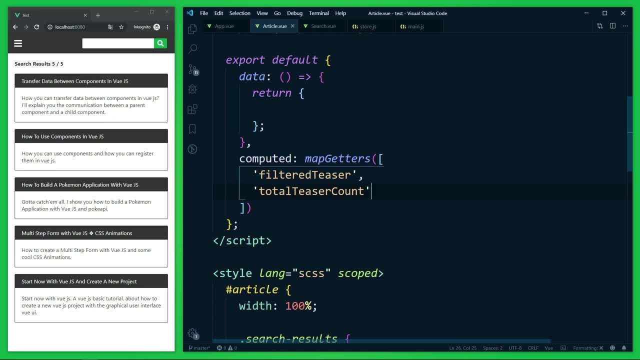 But we have a solution, thankfully with ES6. Let's put mapGetters inside a new JavaScript object here. But this will not work, because mapGetters on its own creates an object with all these computed properties, which are methods. 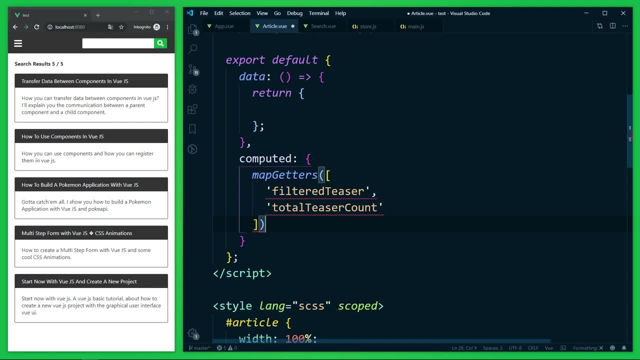 Therefore, you have just an object, which then immediately has a new object. And this is not a good thing. It's not a good thing. It's not a good thing. 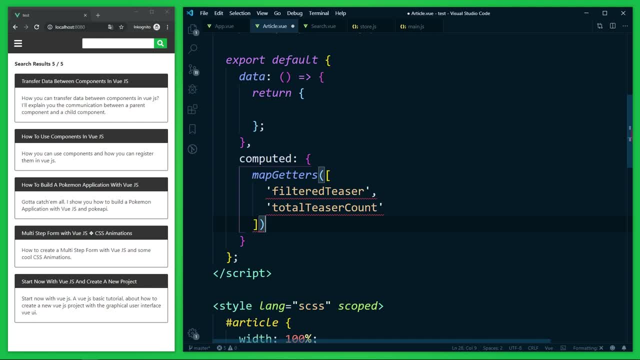 It has an object in itself. And this is not valid code. 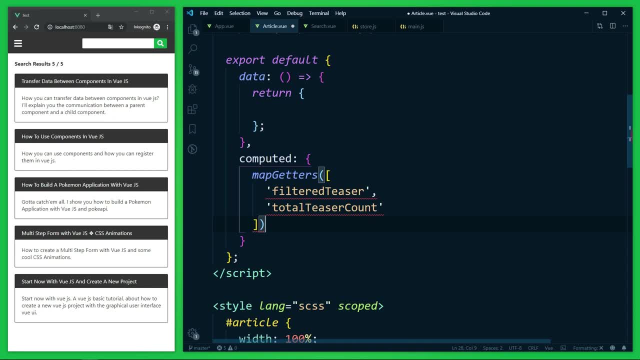 But with ES6, we get a spread operator with these three dots here. This allows us basically to tell JavaScript, please pull this object out and create separate key value pairs for each item of them. 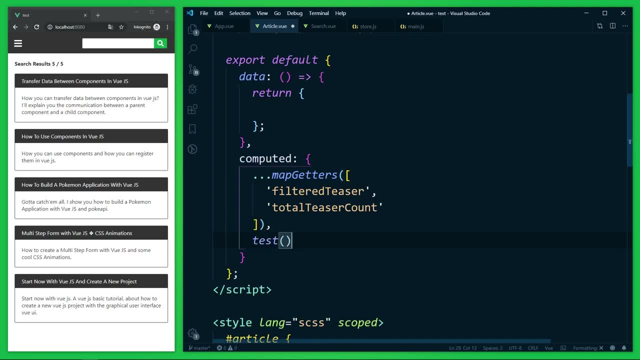 With this, you can now add your additional computed properties here, like this one. And have no issues anymore. 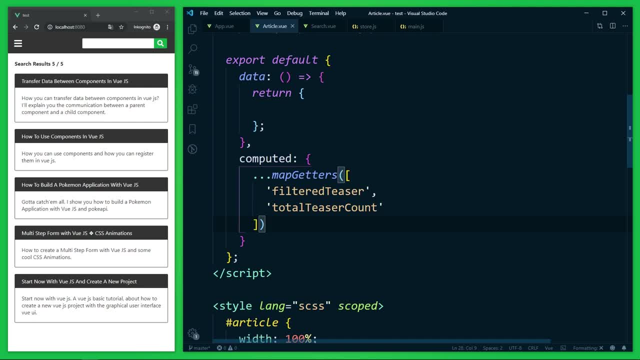 Now this is a great way you can use getters as computed properties and mix them up with others. 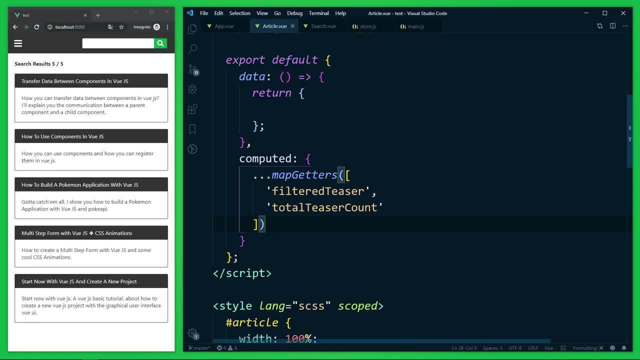 Ok, time to take a look at the infographic again. 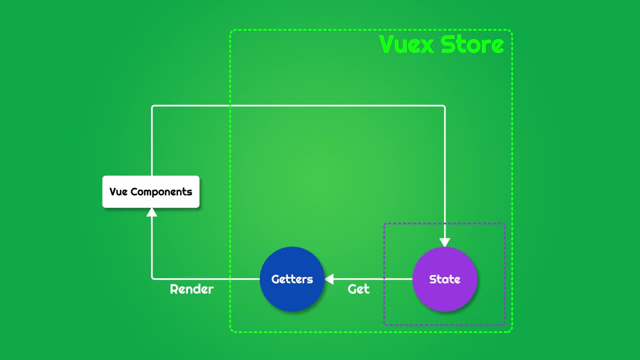 Basically, you could have the same problem if you change your centralized state directly in your components. It's hard to track again. 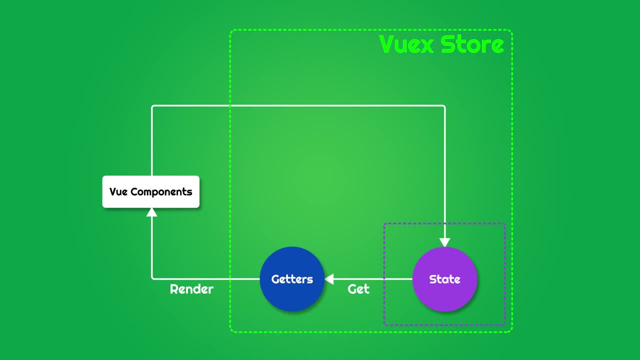 Each component changes your UX state if you use multiple components. 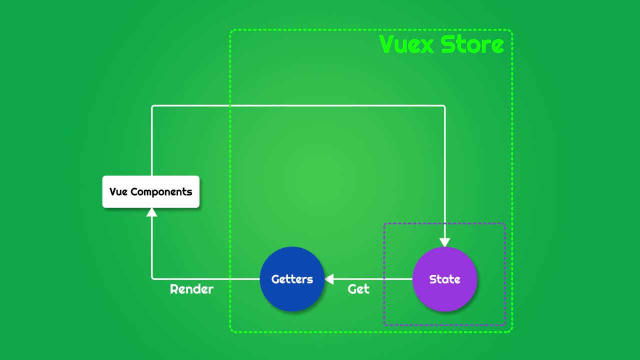 And you would quickly face the problem that you have duplicate code again. And therefore, that is not really the way we want to go, especially not in larger applications. 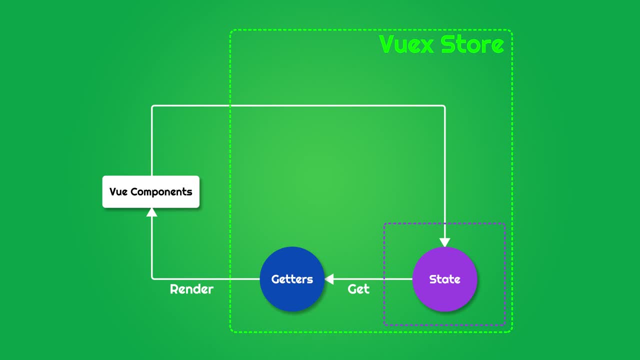 So the solution is to use a similar concept as with the getters, but now for setting the values in the centralized state. 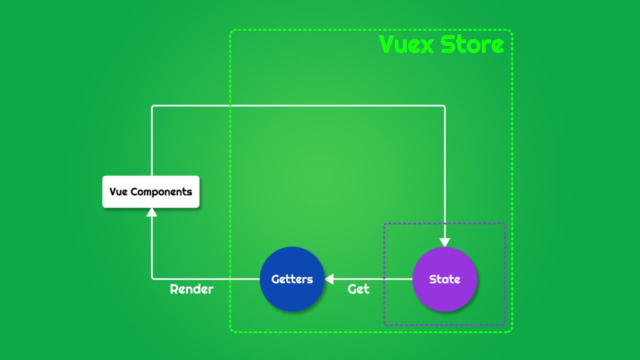 And UX provides a new property. For this called mutations. Because it mutates the state, it changes the state. So you basically commit a mutation from your component, and then this will update the state, 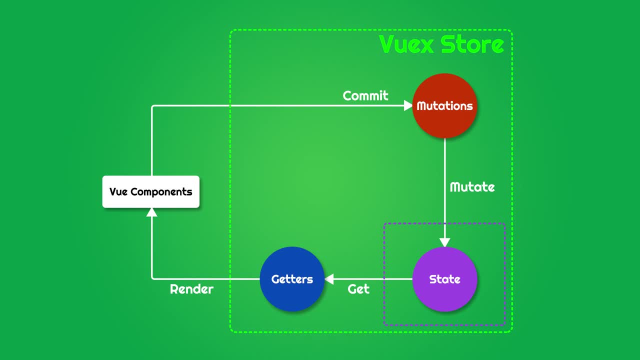 and all the components listening to a getter will automatically receive the updated state or the updated calculation or filtering on it or whatever. Ok. 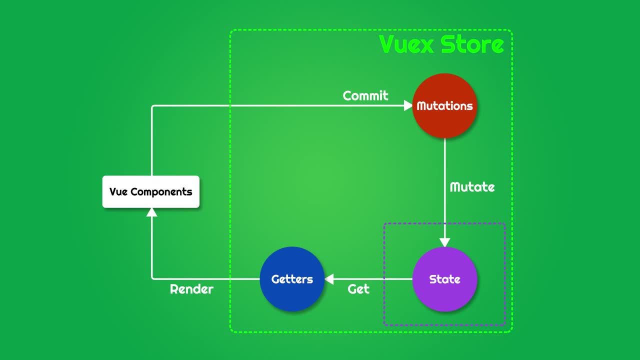 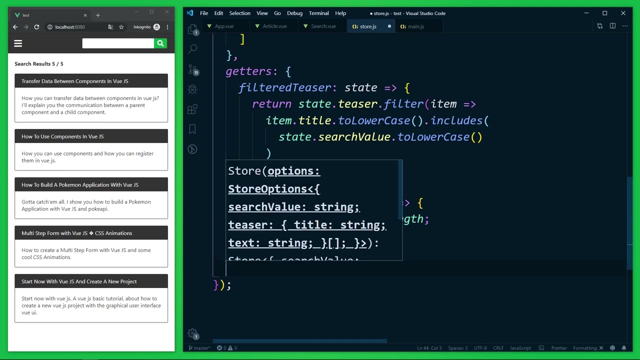 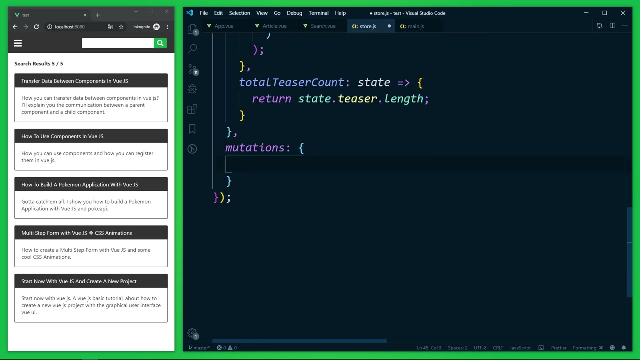 Let's see this in action and see how you can add a mutation. I'm in the stored.js file, and here you can add the mutations property, which is an object, and here you can now create your own setters. Let's create one for the search value we have in the state, for example, setSearchValue. And this function gets the state as the first object. Ok. Ok. So as an argument, this is passed by UX. 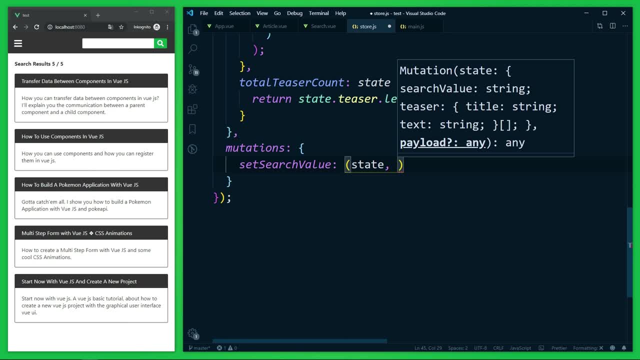 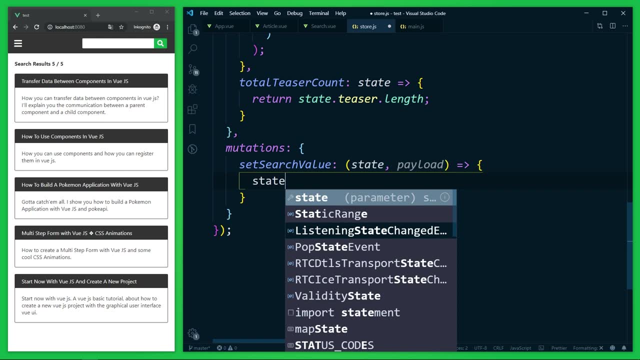 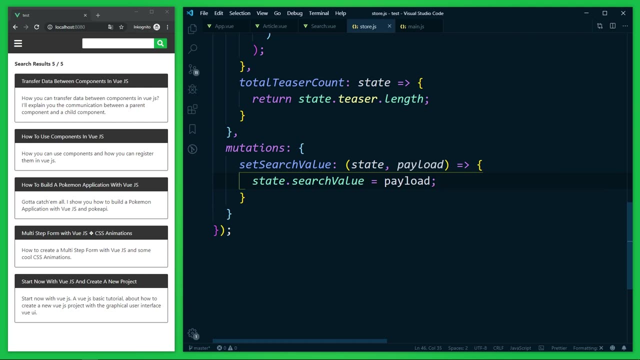 And as a second argument, the value you get from the commit, I named it simply payload. And here in the function, you can set now the state searchValue to the new value payload. 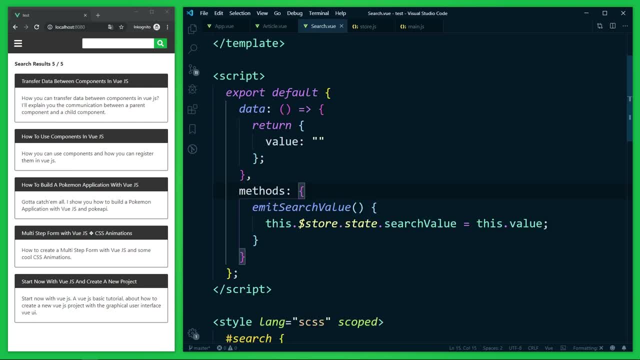 Ok let's stick to the search component, to the emit function here. Where. 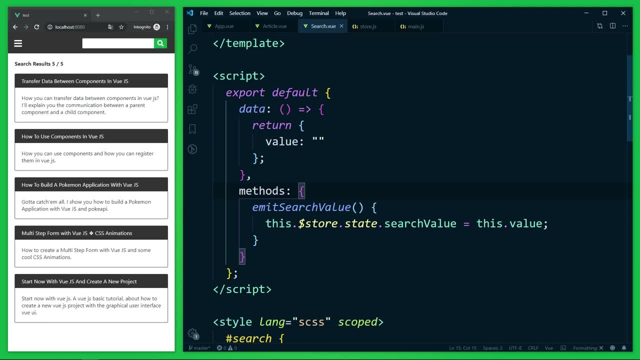 I set the new search value directly in the central state. And here I want to use the new mutation right now. You can do this with this $store and now with commit, which is a function. And the first argument is the mutation you want to commit, in this case, setSearchValue. And the second argument is the new value. 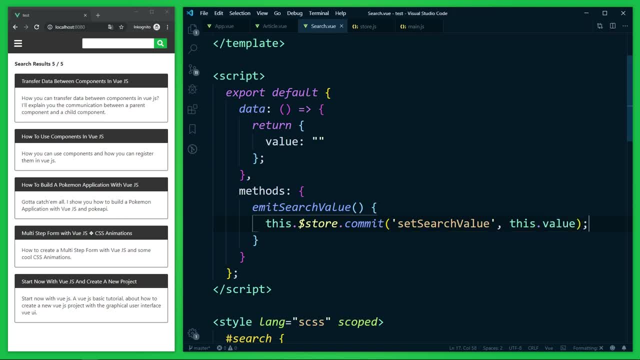 The payload you want to send. That's it. 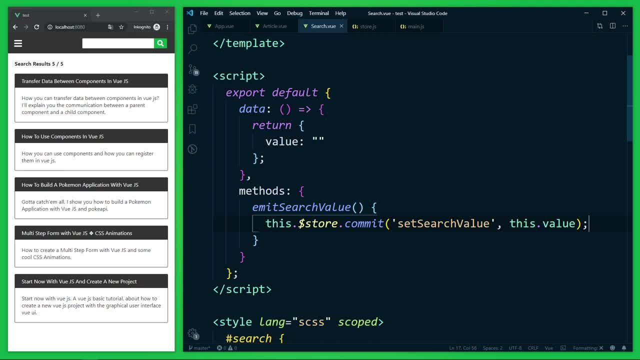 Time to save and let's see if everything works as before. Yes, looks good. 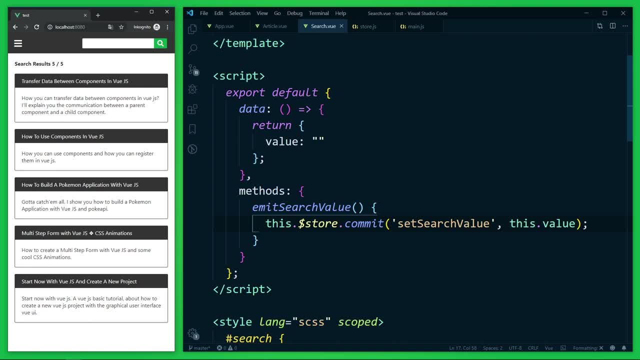 Now if you are creating more and more mutations, then you have here the same issue as with the getters, namely the issue you are repeating this code here over and over again. 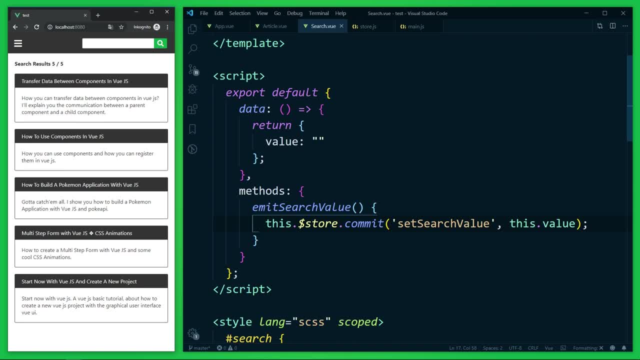 So turns out. UX provides a helper function, similar to MapGetters, and it works exactly the same way. 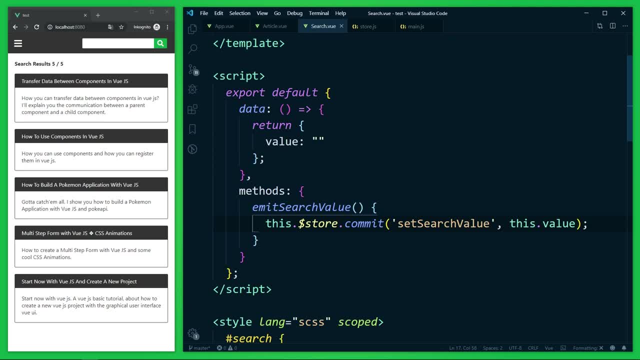 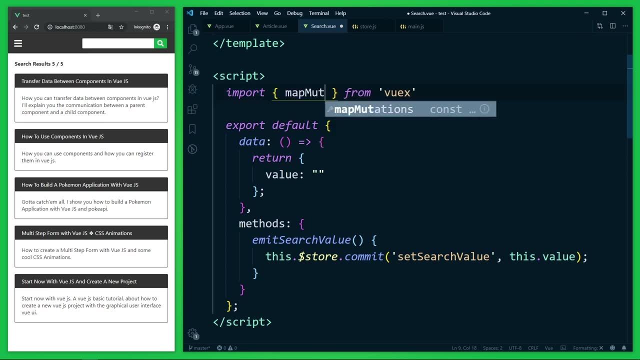 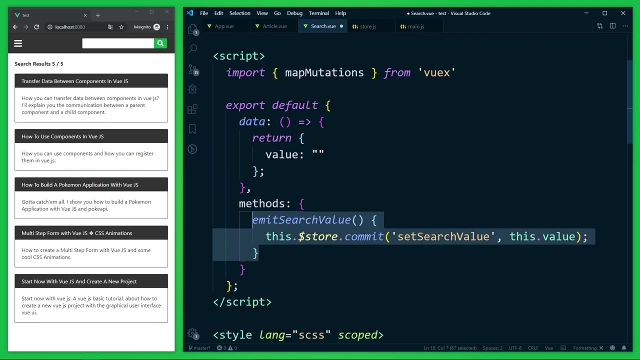 Let me copy this line here quickly and import it in the search component. But instead of MapGetters, you need now MapMutations. And then you can either replace your method with MapMutations, or you remember, the better way is to use the spread operator. The three dots here. If you want to mix them up with other methods. Now as an argument, can you use an array again? Or in this case, I want to use an object to map the setSearchValue mutation to the local function emitSearchValue. 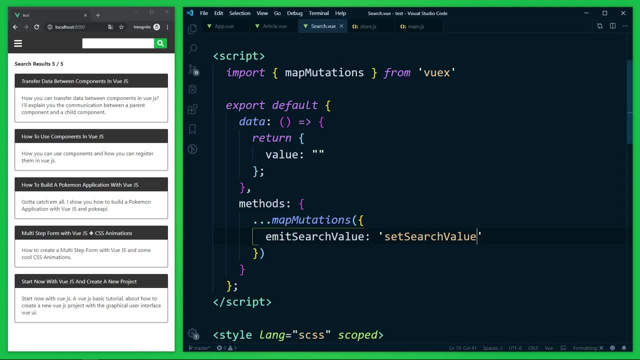 But you can't here set the value as an argument. One solution is to do that. And that's it. 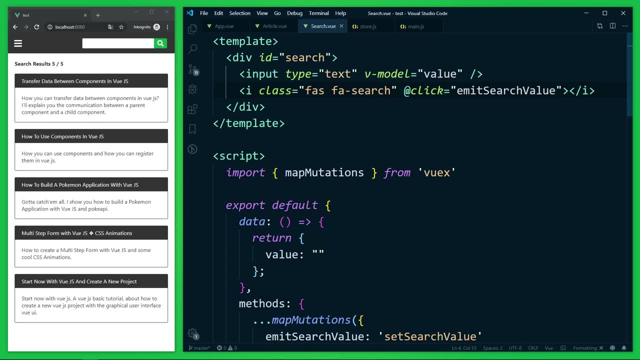 You can do that on the click event here in the template and pass the value. So like with getters, you have now centralized all your changes in one place. And you get easy access to these mutations by having the MapMutations helper. 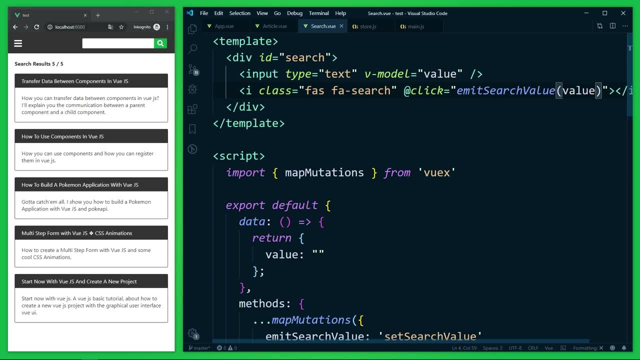 What a great improvement. Or maybe not? 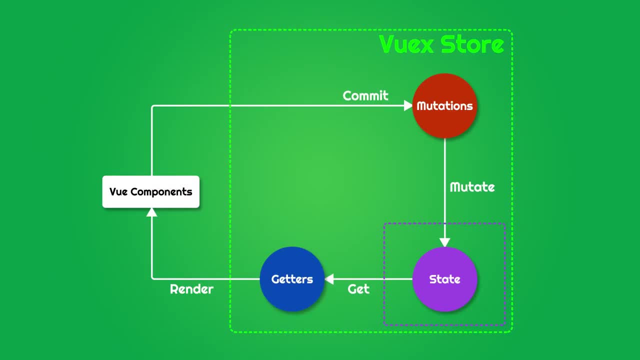 Hmm, let's take a look. There is an issue, a big issue, or maybe not. The problem is that all mutations are only run synchronously. 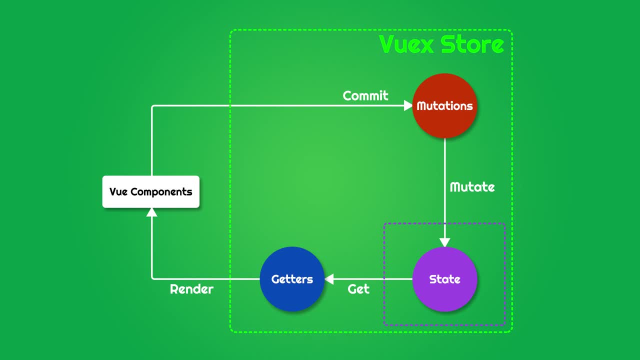 That means you can't run any asynchronous task in such a mutation. So if you want to set a timeout, or let's say you want to reach out to a server to get or send data with your backend, this will not work. 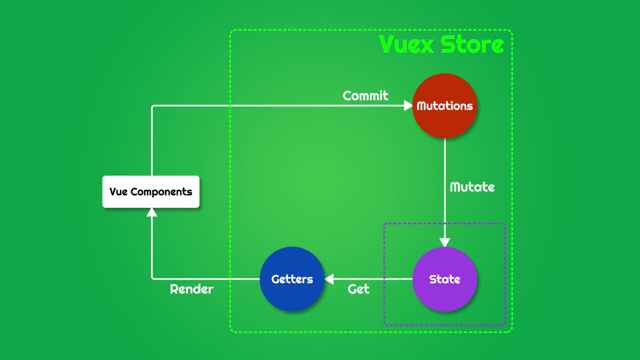 But on the other hand. You need to set a timeout. You need to run the synchronous task, otherwise you can't track any change on your state. Because your state can be changed from every component and you can't tell if the order of changes matches the order of mutations. Because some mutations might take longer than others. So that is a big problem. 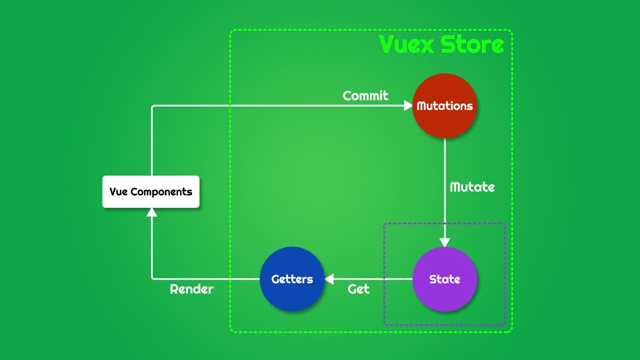 On the one hand, you want to have this reliability by knowing when you make a commit, this changes the state immediately. 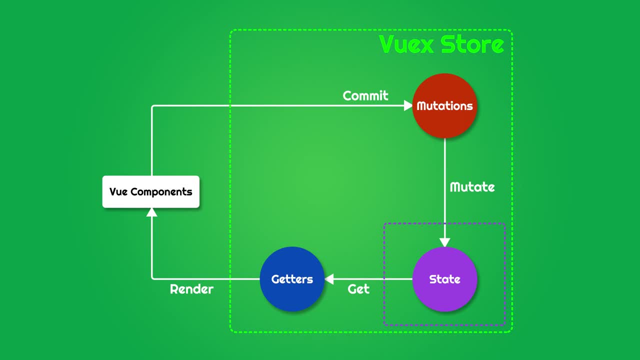 But on the other hand, you also need the functionality to perform asynchronous tasks like an API call, for example. 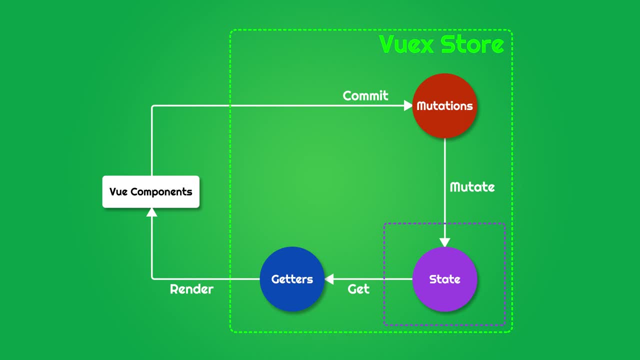 So how you can combine both asynchronous tasks with mutations? Now Vuex provides another property for this called actions. 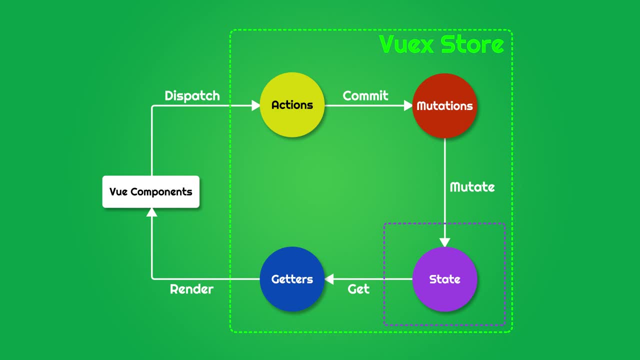 And an action is basically a function where you may run asynchronous tasks and commit one or more mutations with this task. 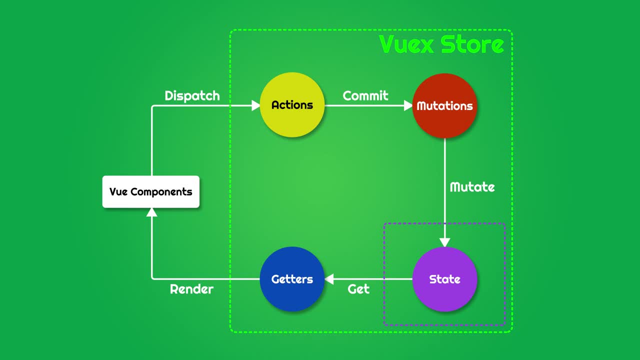 If this task is done. And this is a major benefit. You can use Vuex now as a separate data layer between your backend and frontend. To send your data, to fetch your data and to make some changes or calculations on your data, centralized and decoupled on one place. 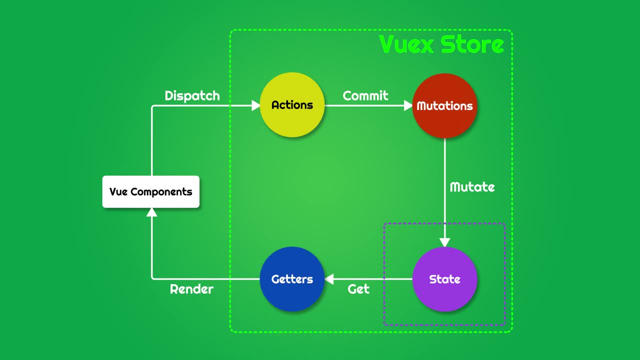 You may trigger an action in a component, you dispatch it, then you send a request to the server. It takes a couple of seconds. And no changes are committed at this time, the state has not been changed yet. 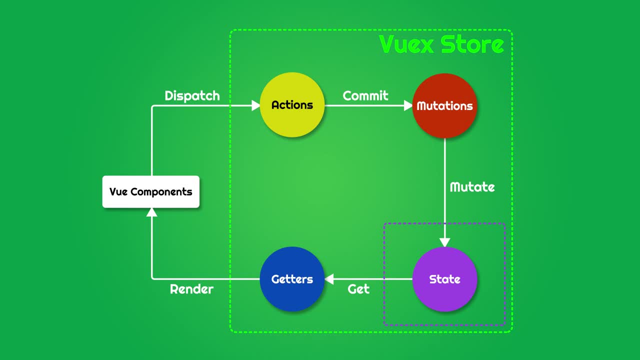 Only if the request to the server is finished this point of time, then you commit the mutations and change the data in the store. You are still able to execute some async code before making some changes. 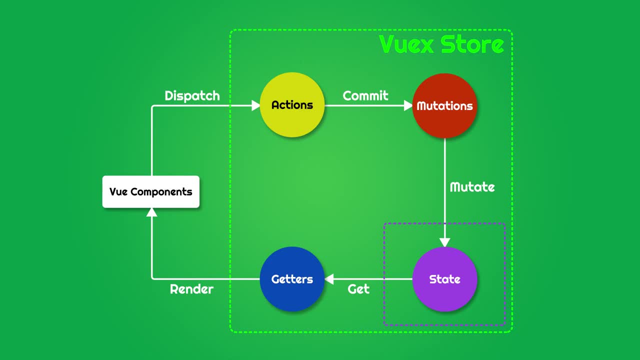 Well, let's see these actions now in action. 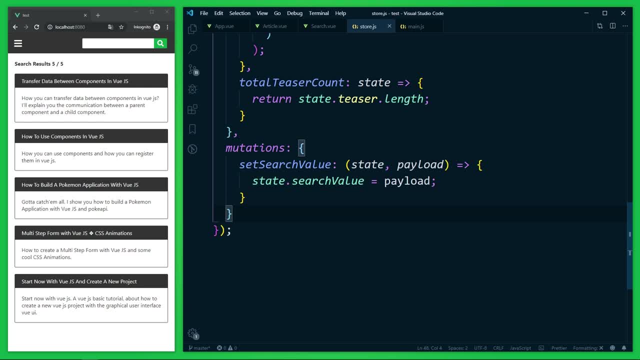 Okay, back to the store.js file and let's use our new property, actions. This is a separate object like the others, too. And here you can create your action, methods, search teaser for example. And all actions get automatically passed as first argument, the context. And context basically just gives you access to the commit method. 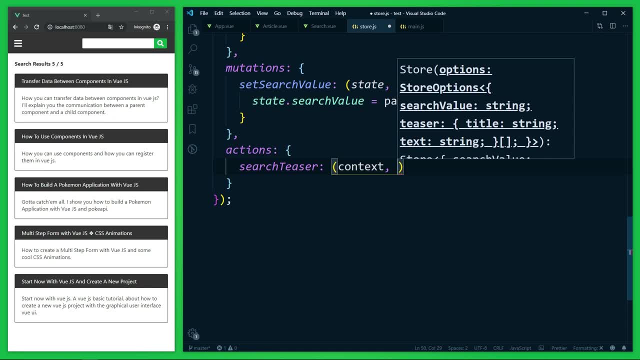 Where you can commit your mutations, here in the end, and as second argument, the payload you can pass to this function. 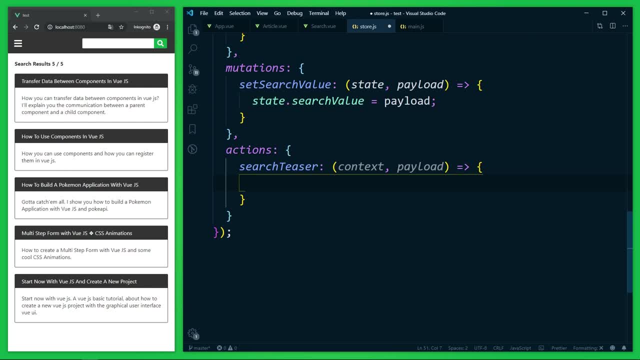 And here you can do some asynchronous tasks. Let's simulate an API call with a setTimeout function. 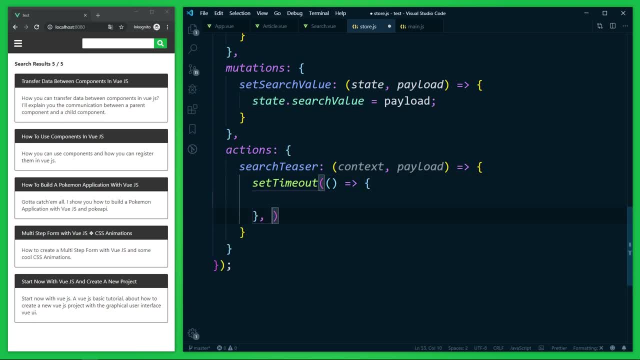 I set here quickly the callback function and the timeout to 2 seconds. Now with context, you have access to the store, in general, just not all features, but to all you technically need here. 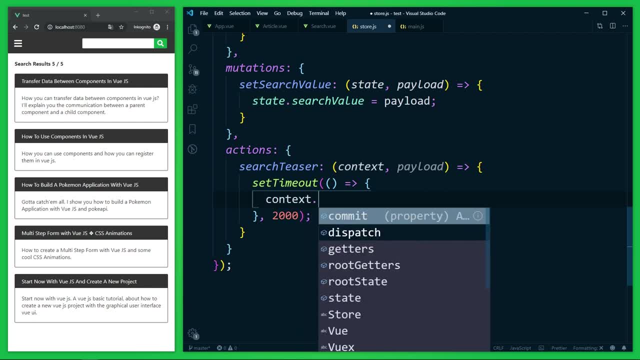 And here, I want to commit now the payload to our mutation. So I write commit, and as first argument the mutation, setSearchValue, and as a second argument the payload. 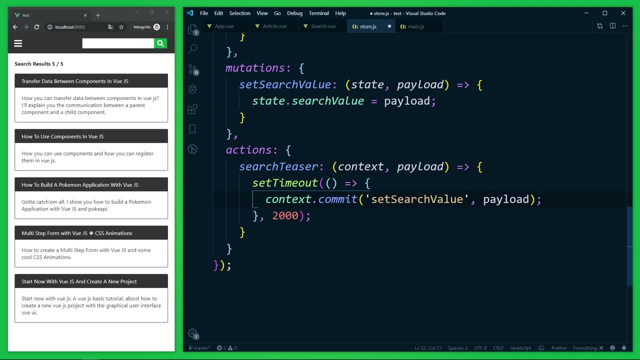 Ok. That looks pretty good, but I want to tweak this function a little bit more with a promise. 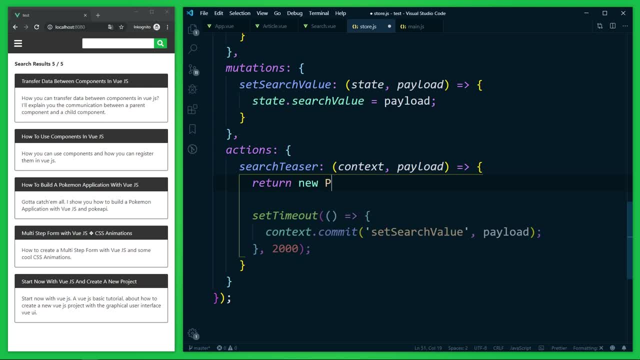 And I want to return it to respond to it later in the component. If you don't know what a promise is, the short answer is, promises in JavaScript are an important feature to greatly simplifies working with asynchronous code. You make an asynchronous request. For example, and wait for a result. And whenever the request is finished, you can continue to work with this result depending on your success or failure. 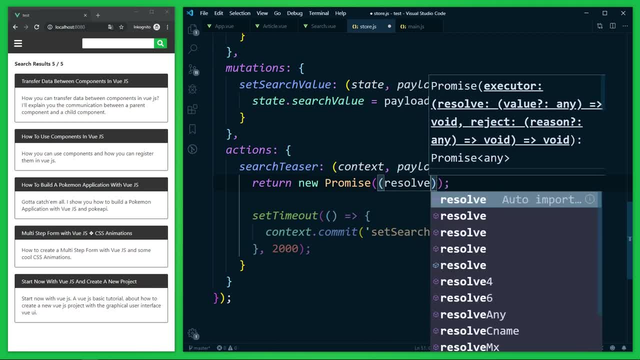 Now here you can set a callback function. And this function gets two arguments automatically passed, resolve and reject. 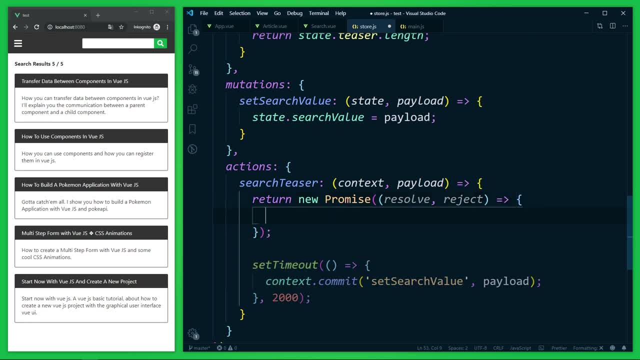 The resolve function is always used if the action is to be declared successful. Reject indicates the result. It indicates that something was unsuccessful. 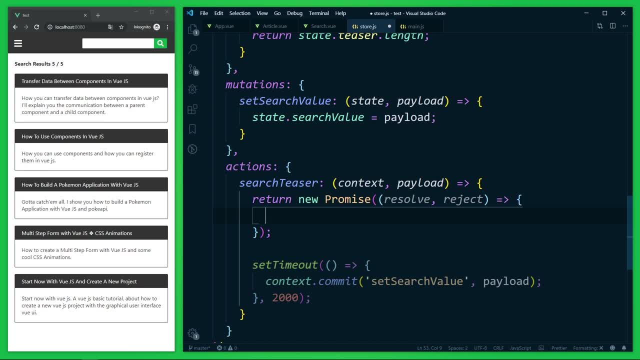 I need only the resolve function, because I can assume that the timeout functions always work. 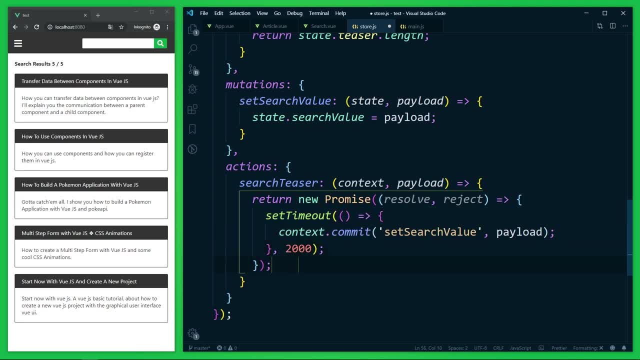 So let's copy the timeout in this promise here and execute the resolve function. You can pass here any data you want. I write simply ok. I think this is enough here. 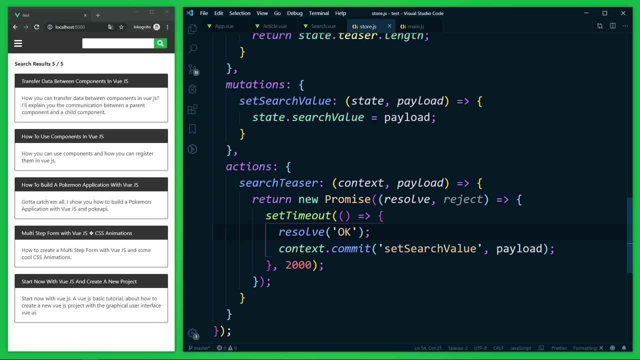 And now you can use this action. Let's stick to the search component, where we use the mutation here. 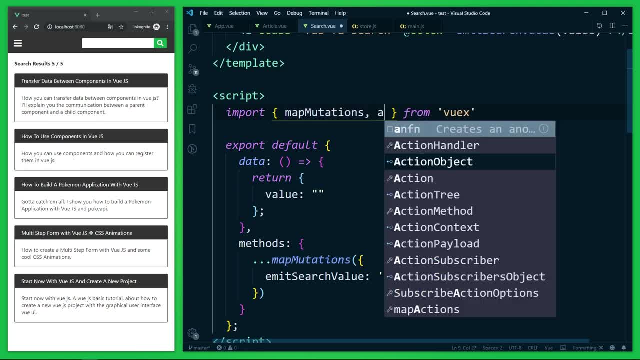 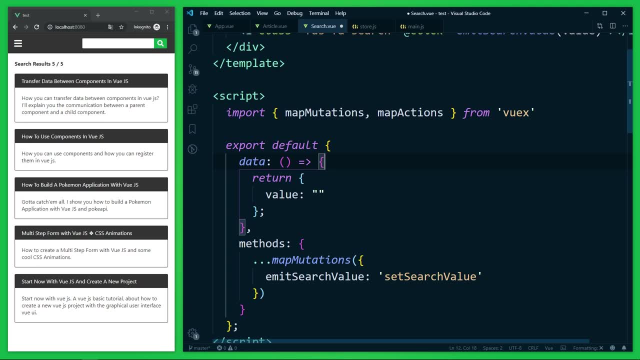 By the way, Vuex provides also a helper function, similar to MapGetters and MapMutations, named MapActions, which you can use here, but in this case, I want to dispatch the action method manually. 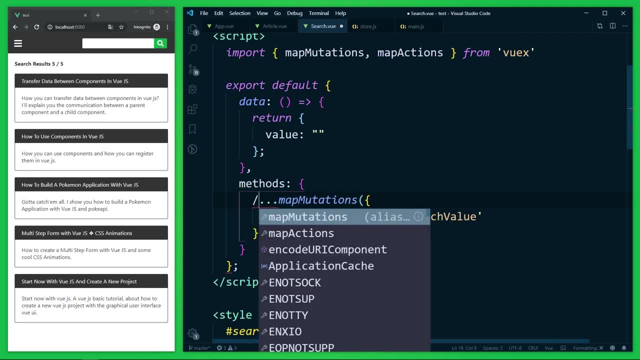 So I comment this here out. We don't need that anymore. And create a new emit function. And here we are. 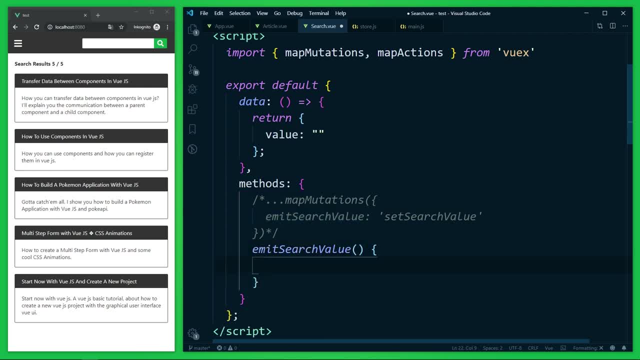 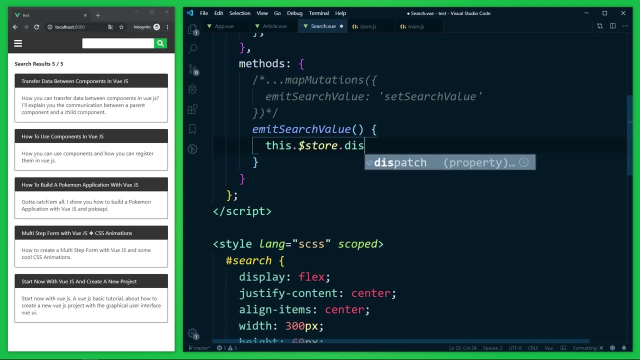 Where you can dispatch the new action method. I do this with this $store and dispatch. And here as the first argument, our action, search teaser, and the second, the value. That's it. And if the simulated request finished, you can use here a function, then, where you can execute a callback function. 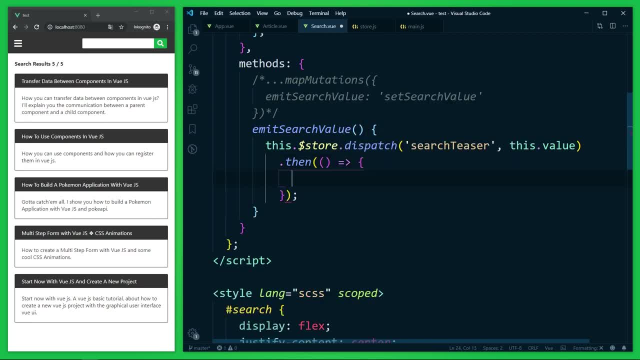 If the resolve function in the return promise is executed. 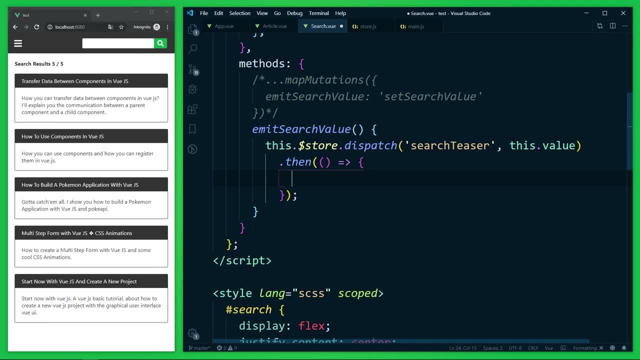 Hmm, what can you do here? I have an idea. 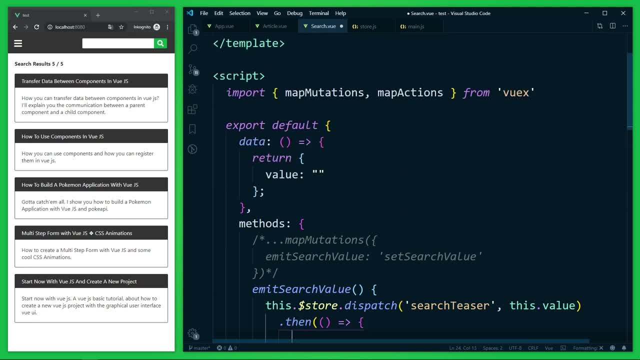 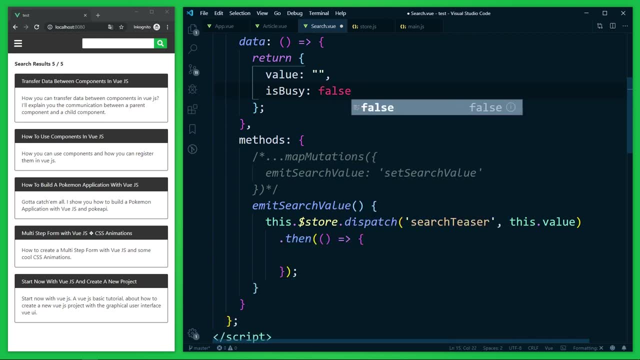 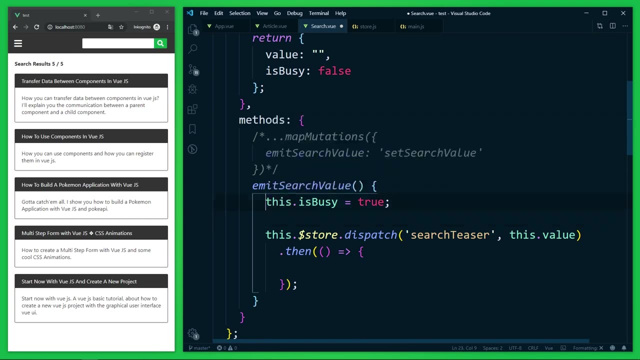 Let's create a simple loader. And for this, I define a status, is buzzy, and set it to false. And when I click on the search button, I set the new status to true, and here, when the actions are finished, I can set the status to true. 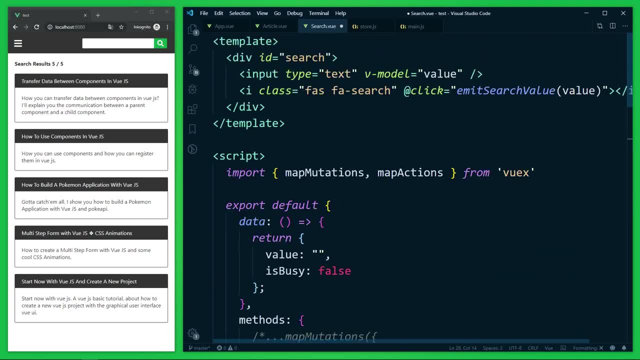 And when finished, I set the status back to false. Let's stick to the template and add a new icon here. I use the spinner icon. 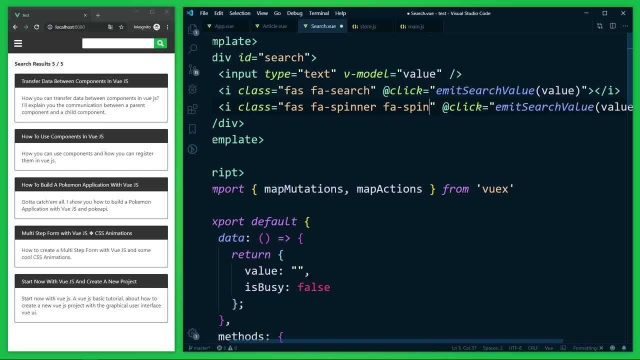 And add also the spin class for the rotating animation. You can here remove the click event. And if the status is buzzy false, then we want to output the search icon, otherwise the spin icon. Ok. 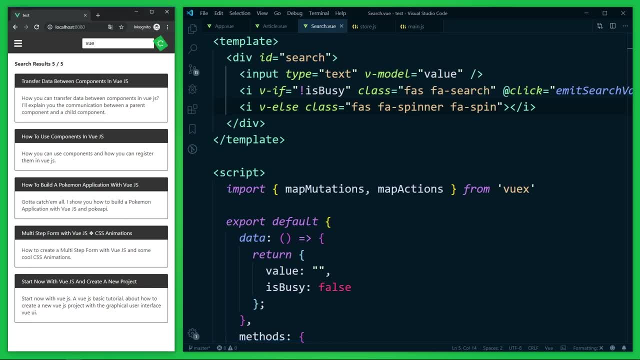 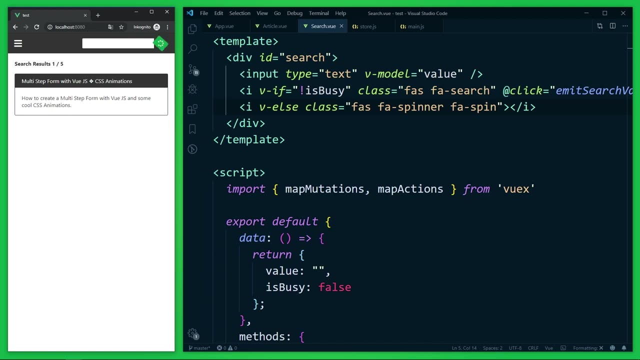 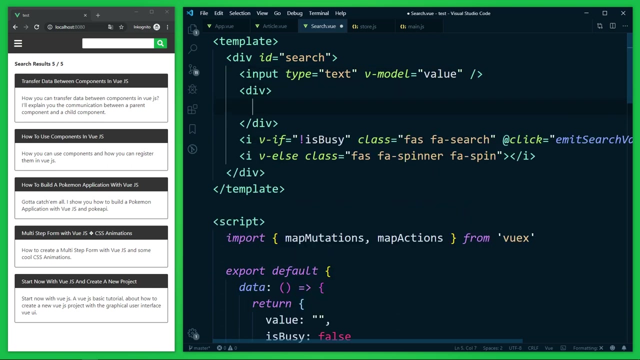 Time to save, and let's see how it works. Hmm, ok, the complete button rotates now. But apart from that, the simulated request works really good. So let's fix this funny button here, by creating a new div around the icons. 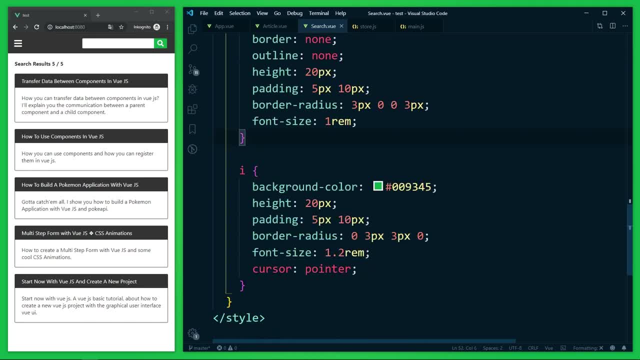 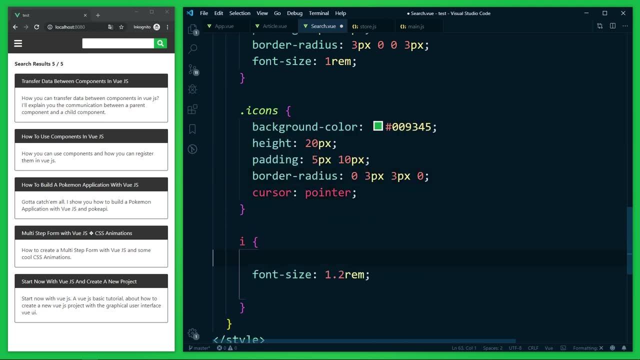 And here, I want to separate the style from the icon element. That should work, I hope. 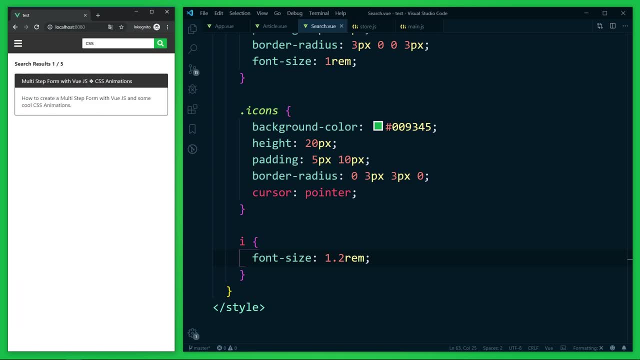 Let's check this. And yes, it looks nice. 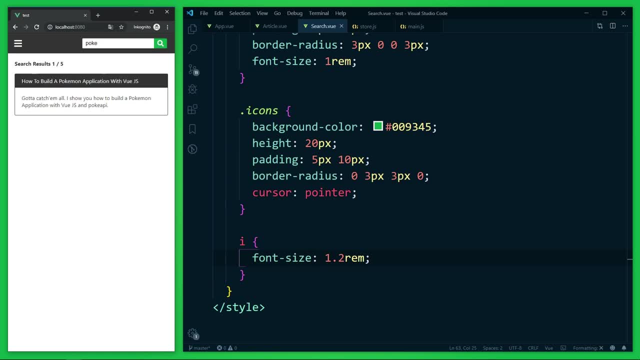 Ok, that was really a lot stuff in one tutorial. But Vuex is, in my opinion, a key feature for loaders.